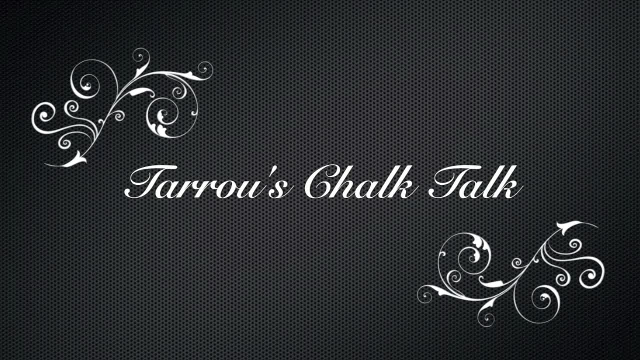 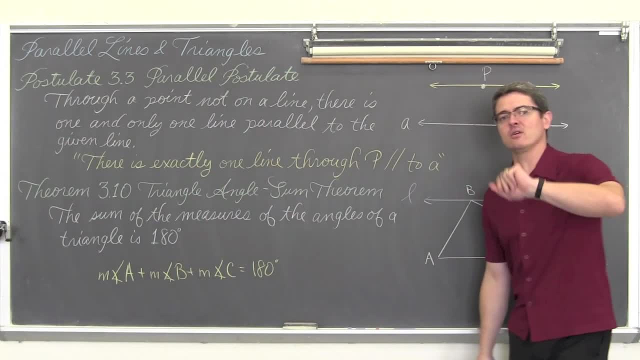 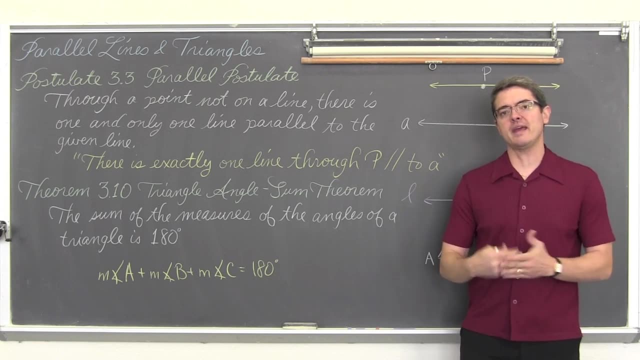 BAM. Mr Tarrou, In this video we are going to be talking about two theorems and a postulate. These theorems are going to be going towards moving into triangles and working with angles that are inside those triangles. So the first theorem is going to be talking about how the 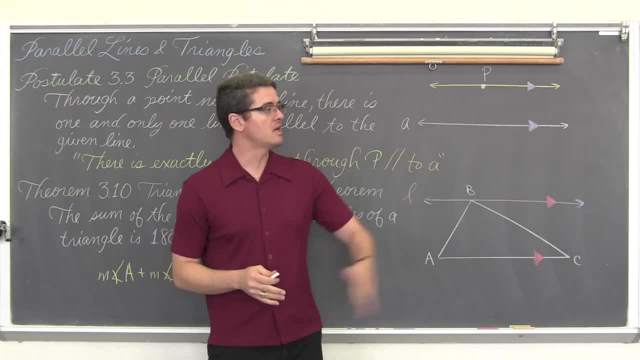 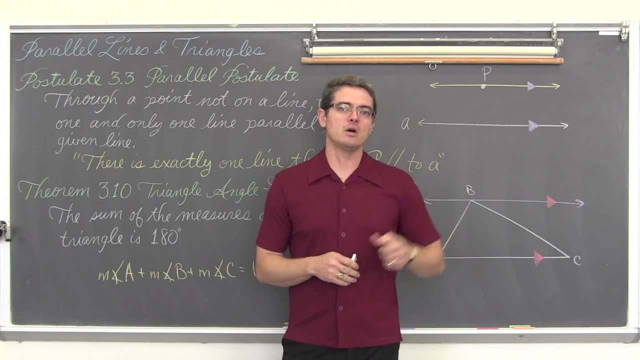 three angles inside of a triangle always add up to 180 degrees. The second theorem is going to be about how an external angle of a triangle is equal to the sum of the two remote angles. So that is what the video is going to be covering today. We are also going to include five examples. 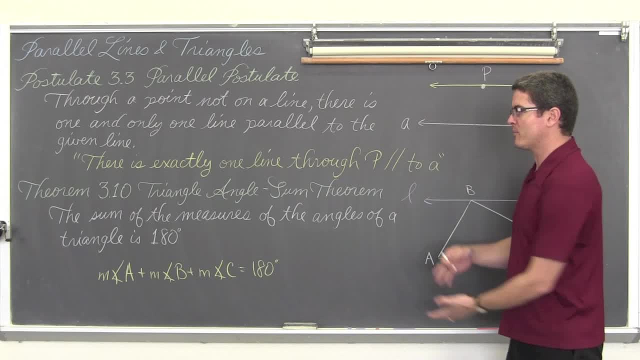 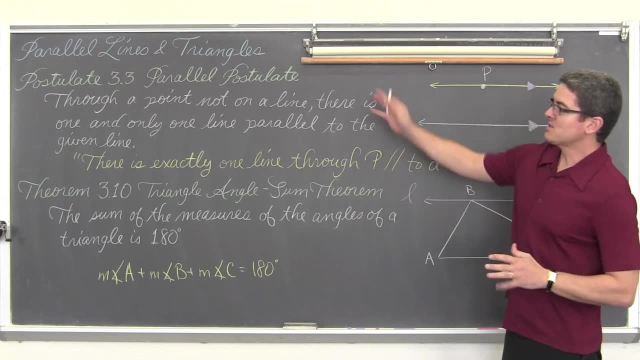 I am going to explain sort of verbally, go through a proof of theorem 3.10, but I am not going to do a two column proof of this theorem. I just want to explain what is going on. So, parallel lines and triangles: Well, the section we are studying is called parallel. 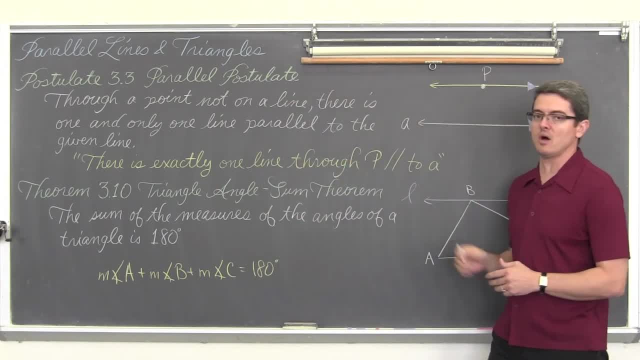 lines and triangles, but the parallel line part of it is called parallel lines and triangles. That part of it is only going to help us explain why the interior angles of a triangle always add up to 180 degrees. So let's start off with this postulate. Postulates again. 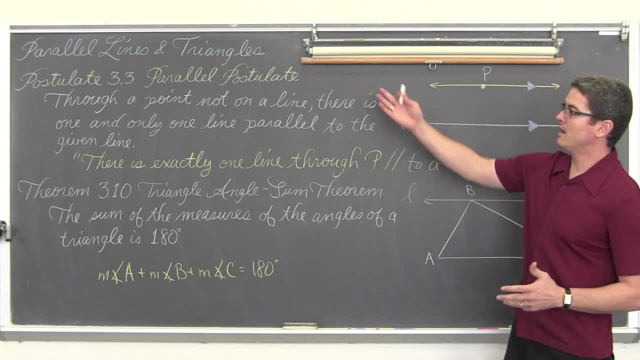 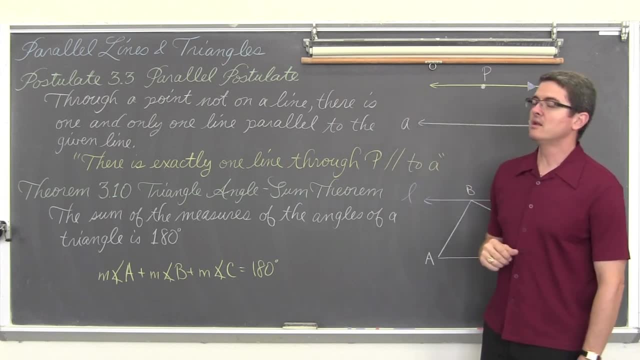 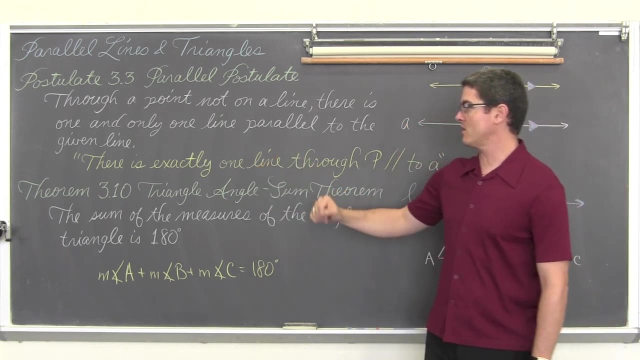 we accept those as given fact. We don't have to prove them. It is labeled 3.3 in my book. but the parallel postulate says: through a point, not on a line, there is one and only one line that is parallel to the given line, Or in other words, there is exactly one line. 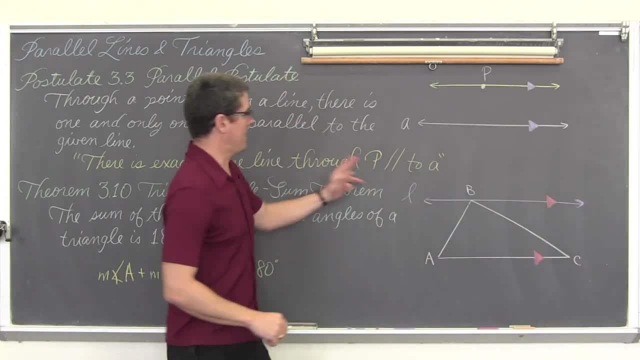 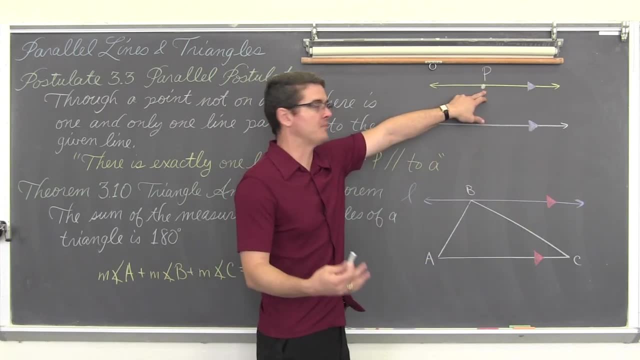 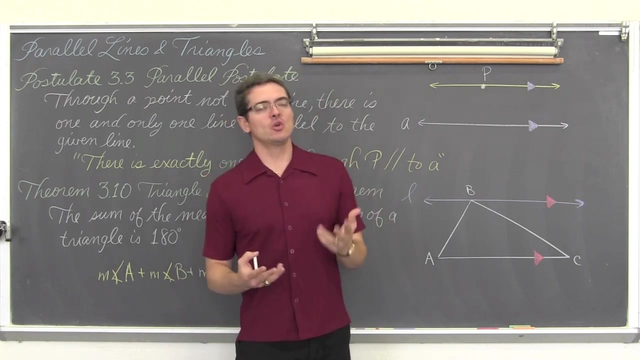 through point P That is parallel to A. So I am giving us a line here of line A. I have put a point somewhere else, not on line A. There is only one possible line I can draw through that point that would be parallel to the given line. So it kind of just not assumed. but we have learned. 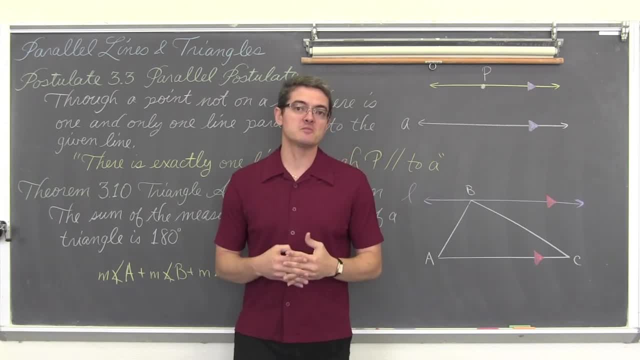 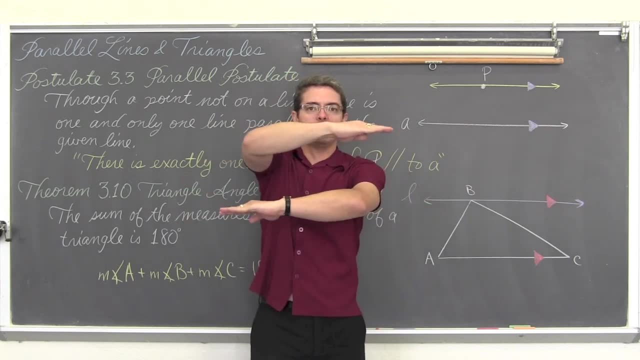 earlier in our studies that two lines that are parallel must be within the same plane. So remember that we. We have this given line A. There is a point out here in space. I am not talking about a skew line, because skew lines don't intersect either, but they are not in the same plane. 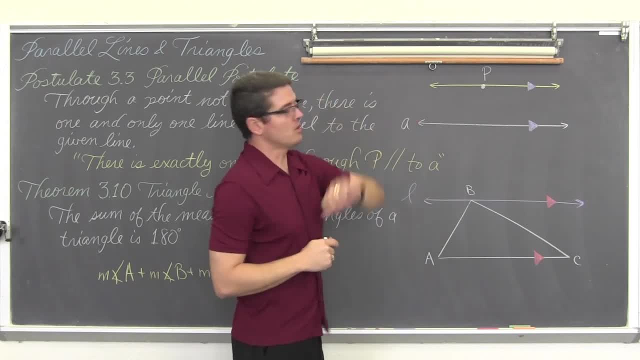 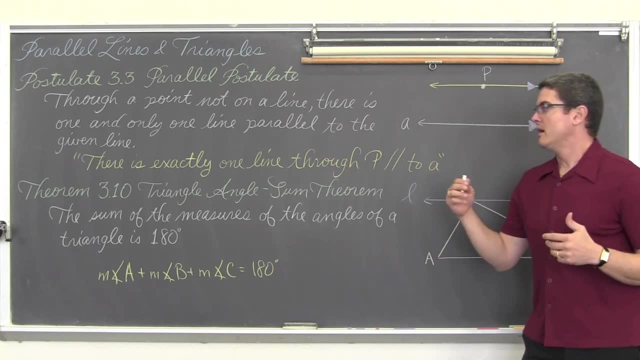 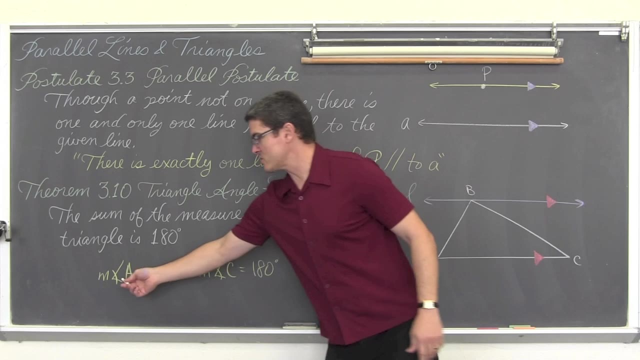 So we are talking about those lines that are parallel. Well, there is only one line that we can draw, Ok. So theorem 3.10 which says: or is the triangle angle sum theorem says the sum of the measures of the angles of a triangle is 180 degrees, Or the measure of each of the 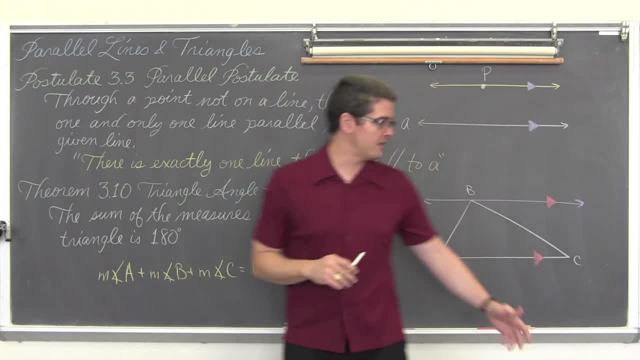 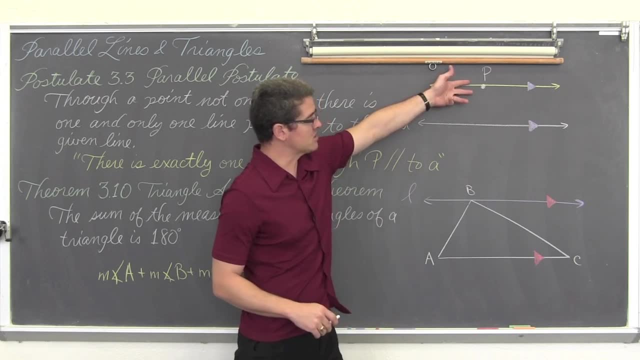 angles added together is equal to 180 degrees. So I have given us a triangle- A, B and C- And I have got a purple line. I kind of like to match up with this yellow line I have up here. I have drawn a line through one of the 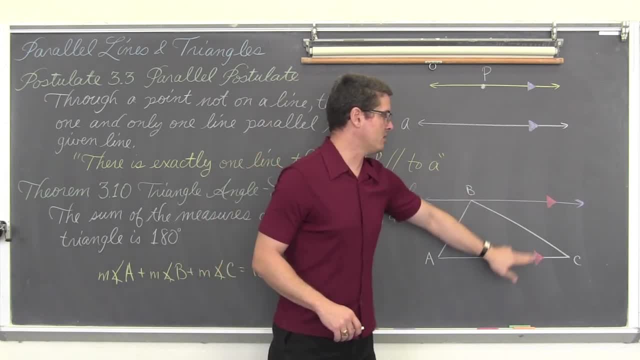 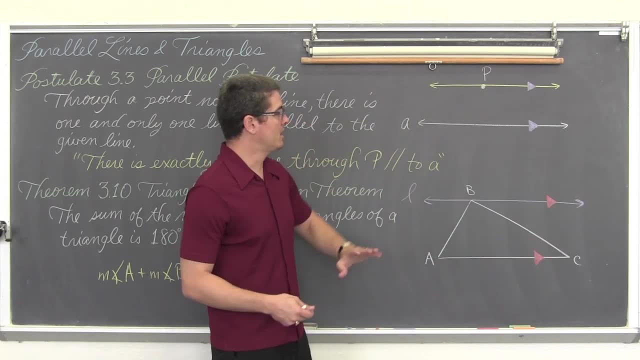 vertexes of my triangle And I have drawn it so that it is parallel to the side of the triangle that this vertex B does not include. So I want to tie in the postulate that I just explained with you And this. I want to tie it together with this theorem and help you. 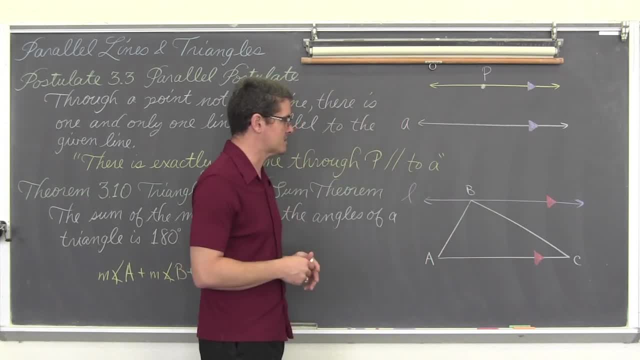 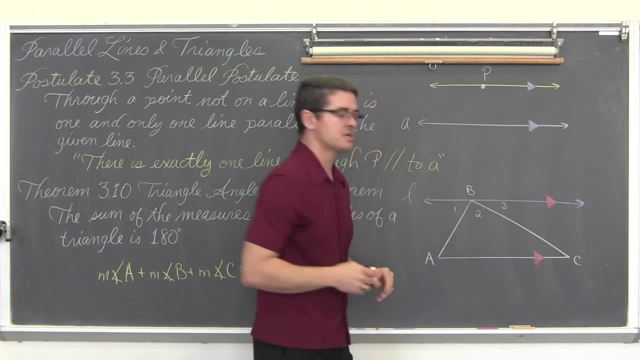 understand why the three angles always add up to 180 degrees. So if I look at the top of this diagram, I have got- let's see here- I have got 1,, 2, and I have three angles that are all adjacent. They all share the same vertex, They all share a common well: 1 and. 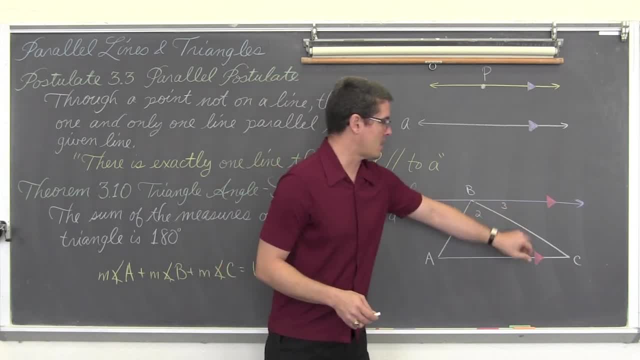 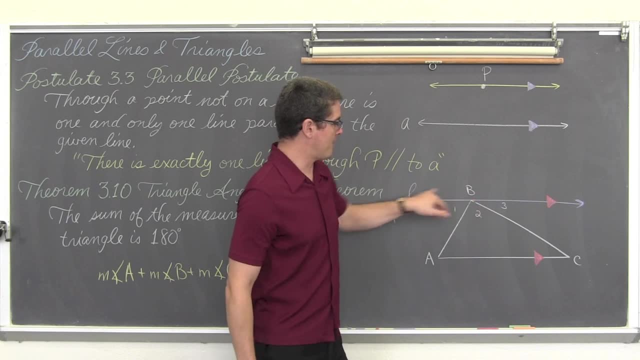 2 share a common side, Angles 3 and 2 share a common side And all of those adjacent angles are sort of forming a line or opposite rays. Remember that rays start from a point and they go in opposite directions, so that there is 180 degrees between those rays. But we 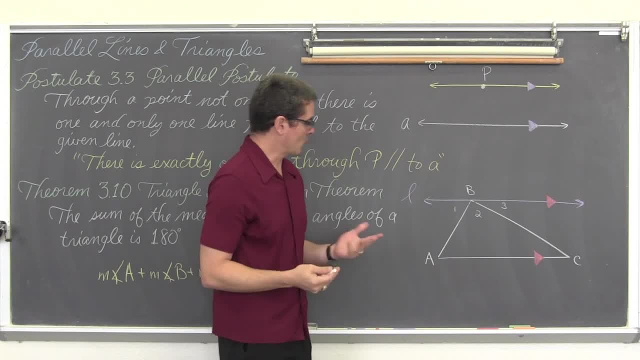 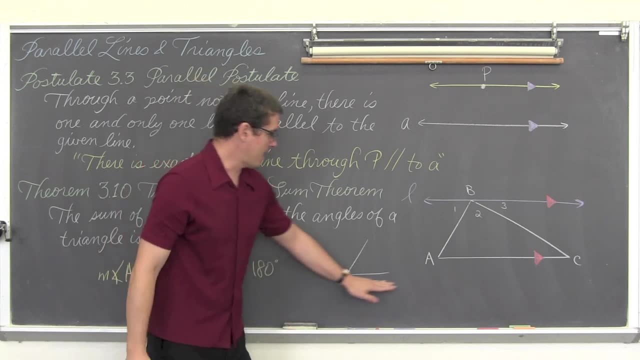 are just going to simplify it and call it a line. Now we have already studied something called a linear pair. We know that when we have a linear pair, we have two angles that are adjacent and whose non-adjacent sides form a line, or opposite rays. And we know 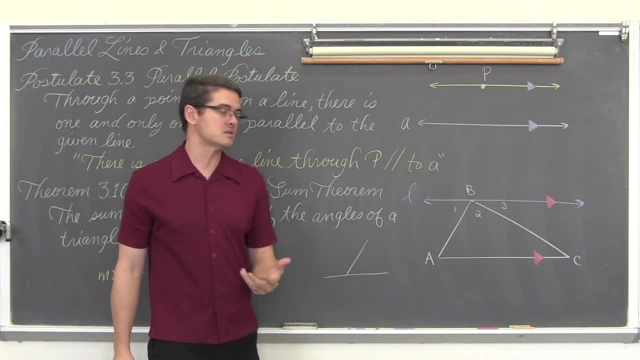 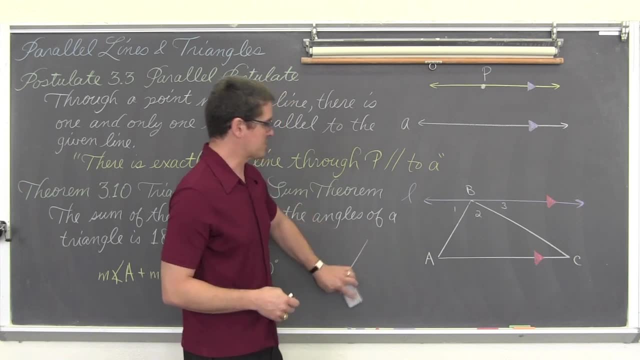 that these linear angles always add up to 180 degrees. Well, I can't call this a linear pair because, well, I don't have two angles, I have three, But I'm going to call this. I guess we call it a linear triplet, but that is not a vocab word in geometry. But these 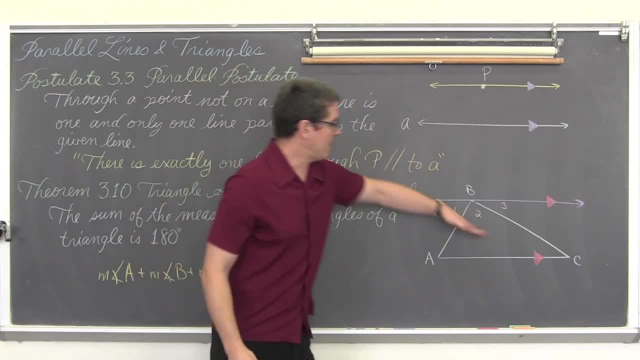 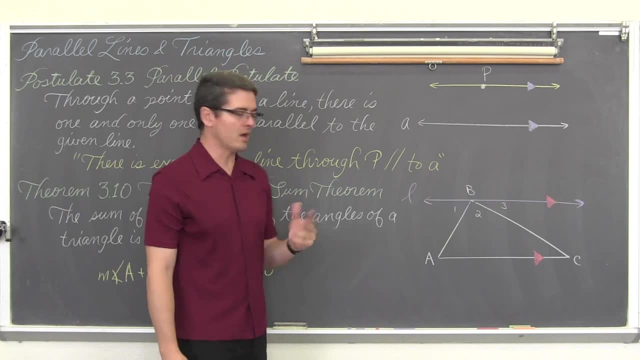 three angles are adding up to 180 degrees because, again, of their non-adjacent sides forming a line, if you will, or opposite rays. So why do I care about that? How is that supposed to help me explain that the inside angles, the interior angles of a triangle, add up to? 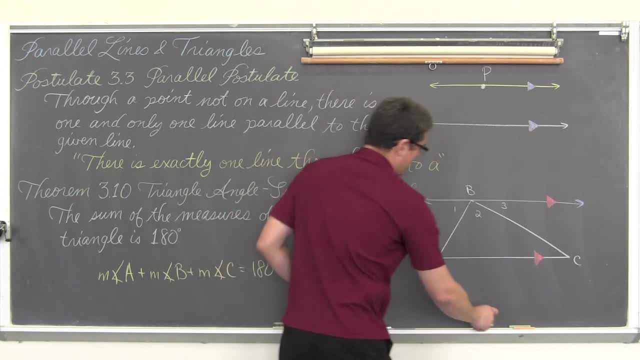 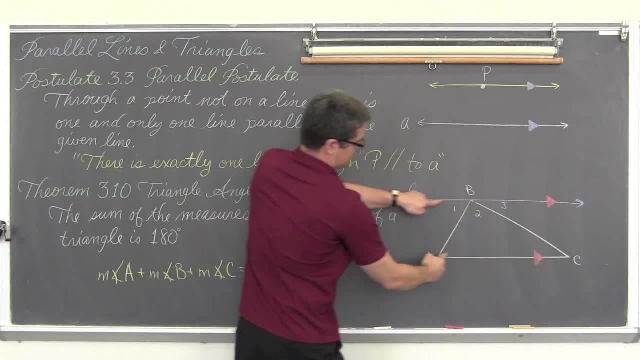 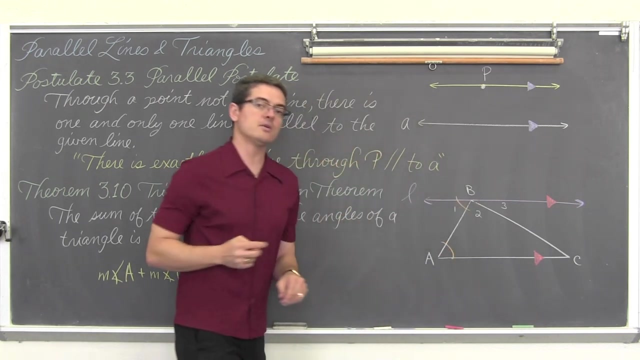 180 degrees. Well, I have got a couple of parallel lines in a zigzag and I am going to use the zigzag area forming here. When two lines are cut by a transversal, My red doesn't show up on camera. let's try this one. My alternate interior angles are going: 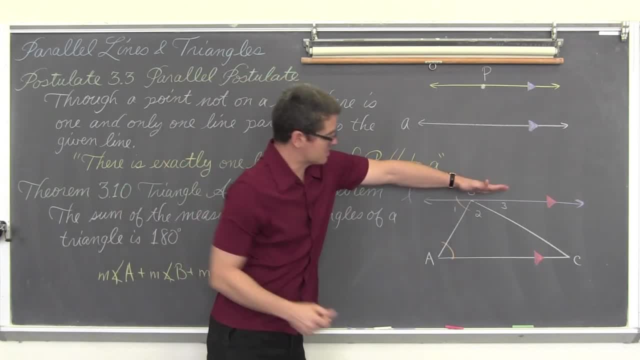 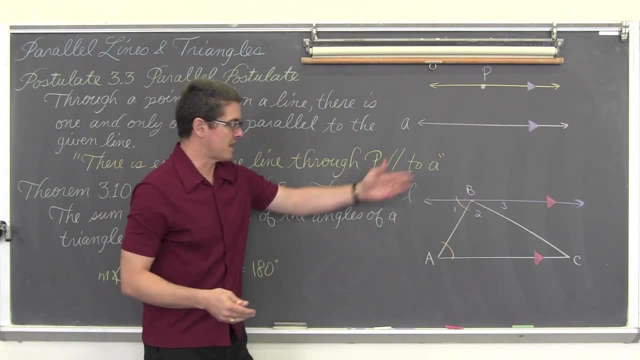 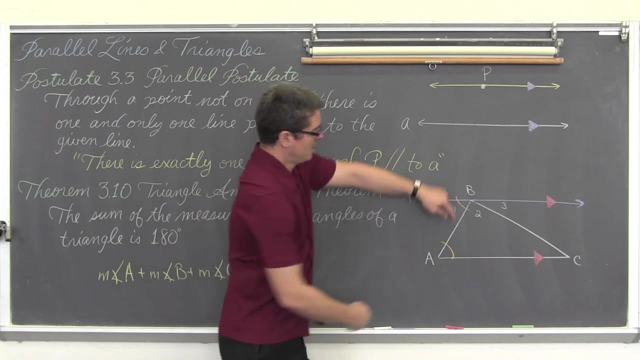 to be equal. So alternate interior angles. when you slice or cut through two parallel lines by a transversal, so line AB is acting as a transversal or side AB or segment AB. since it is a triangle, these sides are stopping at the vertexes: The alternate interior angles. 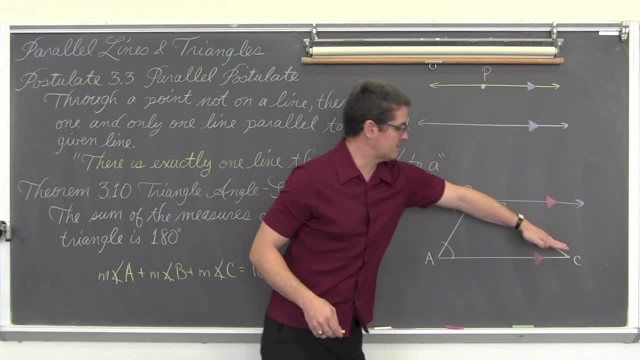 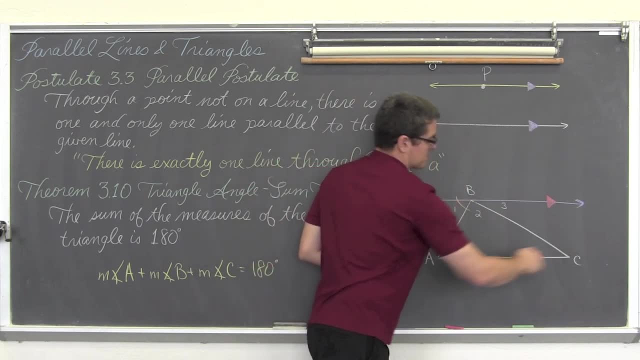 angles are congruent. Well, the same thing is happening over here. I have a different transversal, but again, when I have two parallel lines being cut by a transversal, then the alternate interior angles. you see that z shape, that sort of zigzag shape that is. 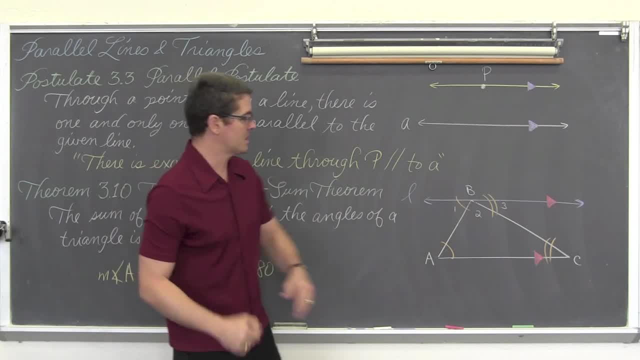 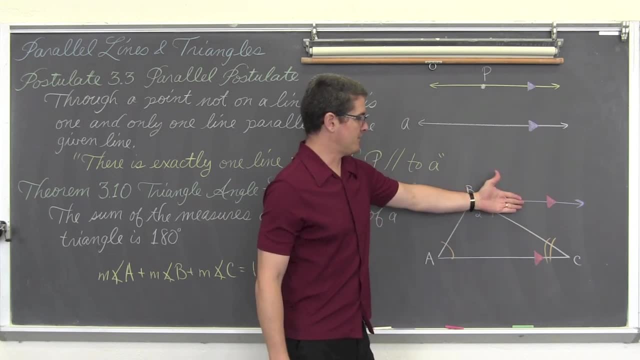 sort of your tell or your give away that you are looking at alternate interior angles. Why are they alternate? One is on the left side of the transversal, or maybe you might consider this below. The other angle is above the transversal and they are both in between. 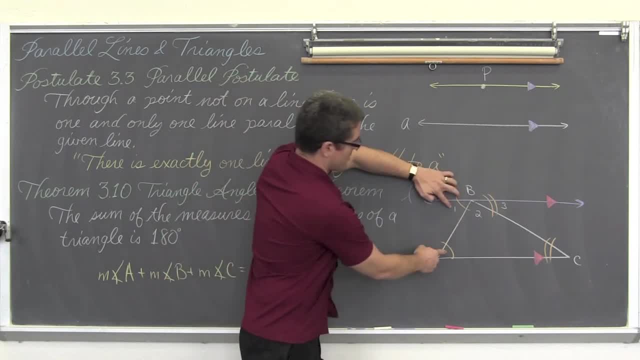 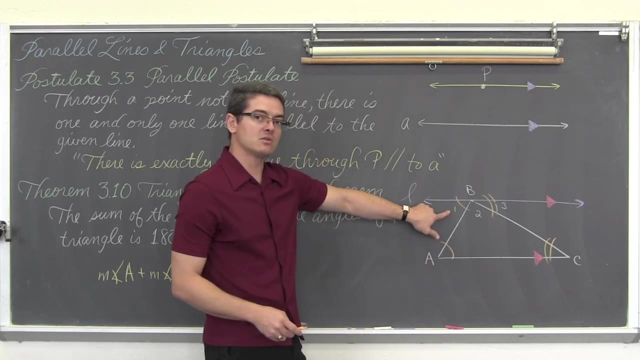 the parallel lines that were cut by that transversal. So again, our alternate interior angles are going to be congruent. So let's see, I had angle one plus angle two plus angle three was 180 degrees. Well, angle A, the measure of angle A, is equal to the measure of angle. 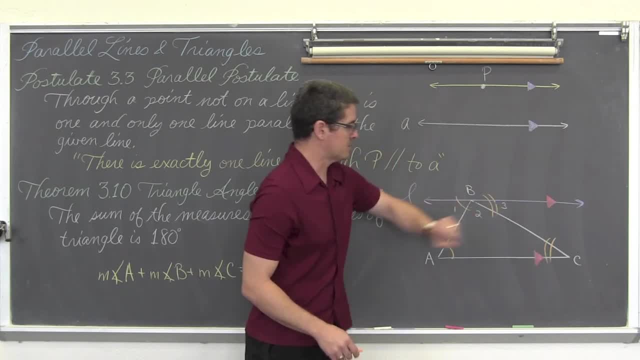 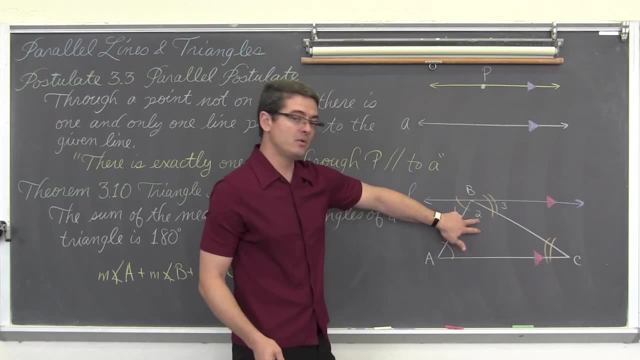 one, The measure of angle C is equal to the measure of angle three, again because of those alternate interior angles. Then we still have the two here Now, kind of verbally, sort of explaining, not doing a two column proof, but one, two, three. 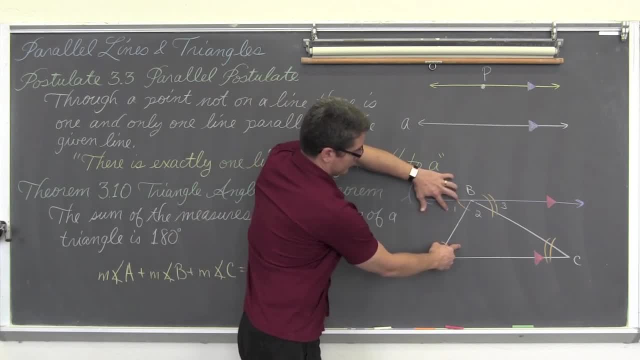 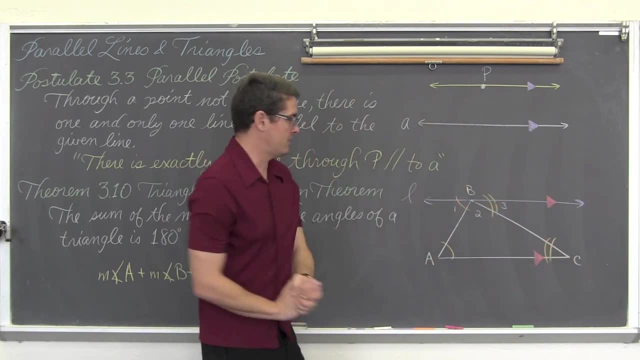 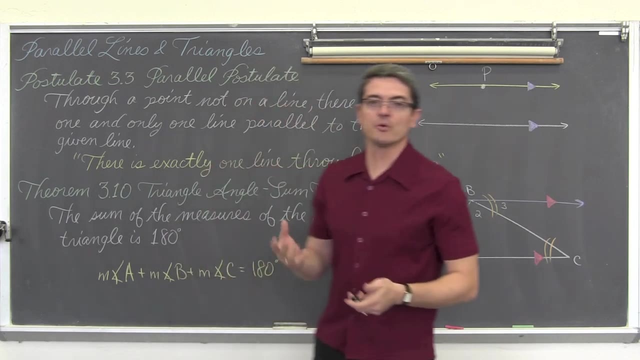 equals 180 degrees. So A plus angle B plus angle C, those are also going to add up to 180 degrees because of this relationship we have here with our alternate interior angles. So that is how we can show or prove that the three interior angles of aof any triangle 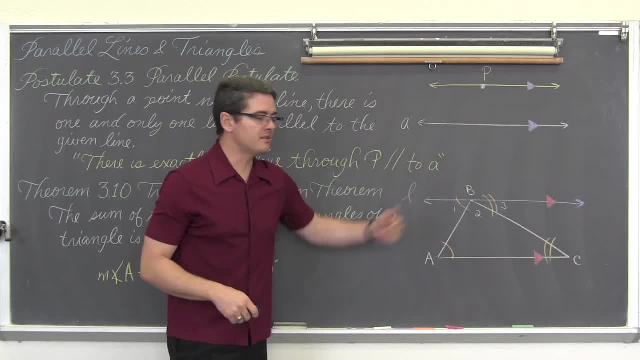 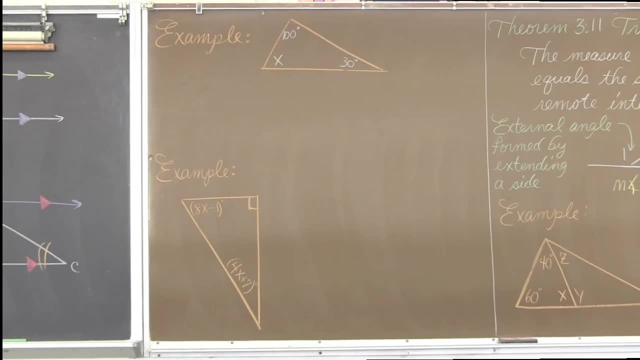 always add up to 180 degrees and 80 degrees. Let's take this theorem, now that we know is valid, and do a couple of examples with it. WHOO, I love this stuff. Here are our two examples. We have an example number. 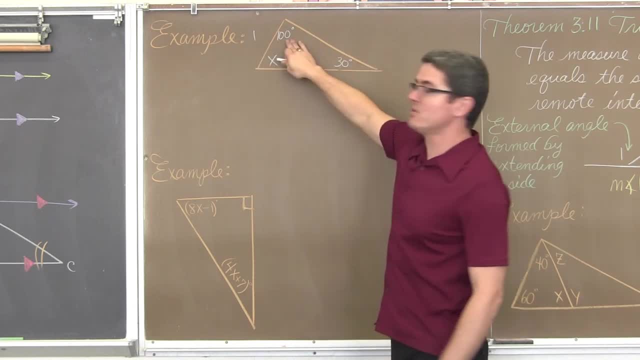 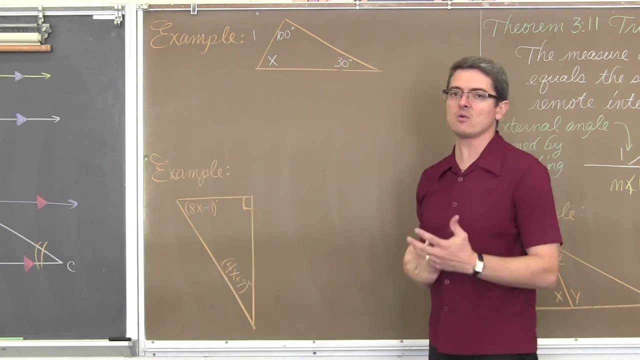 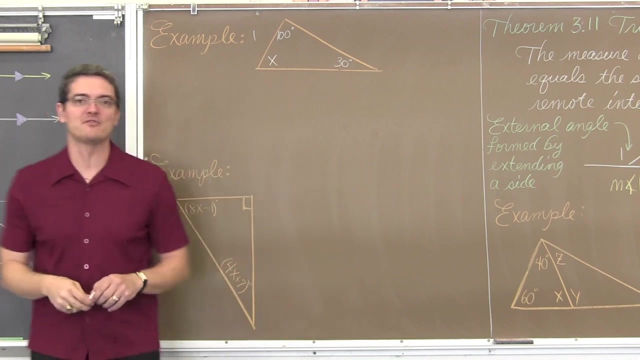 I guess let's call it 1.. So we have an obtuse triangle. We have an angle there that is over 90 degrees. Pretty simple, I have 130 and x. I want to solve for x with both of these problems. We have this little fusion of geometry and algebra that happens pretty often using 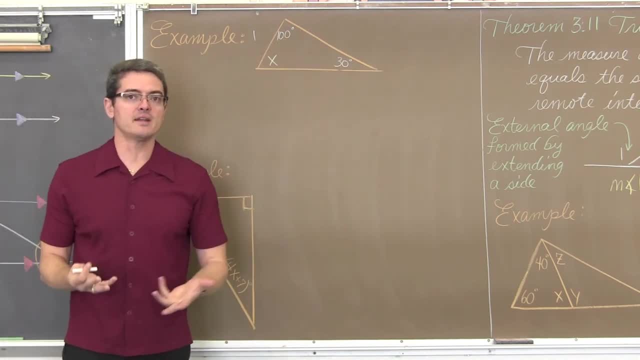 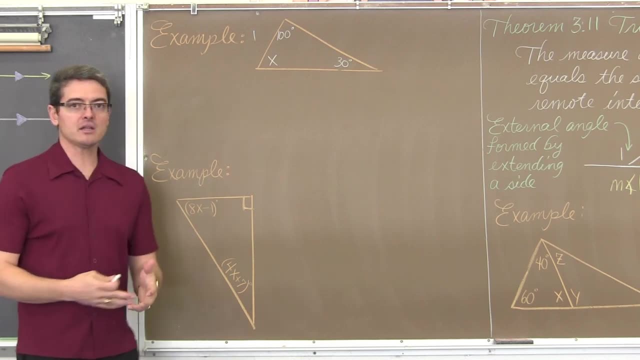 our algebra 1 skills. So we have these three interior angles. We want to find out what x is. We need to remember that the interior angles add up to 180 degrees. Now I can explain over and over again, like I did over here, why that is the case, but now it is going to be. 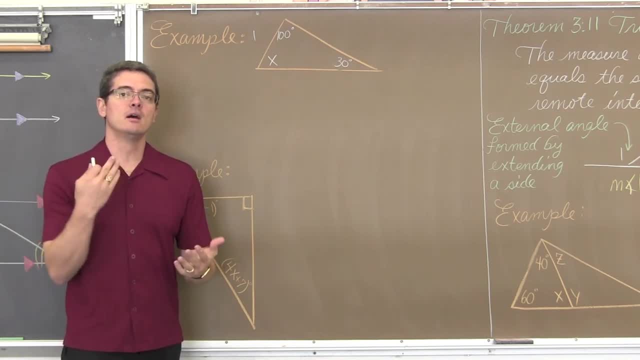 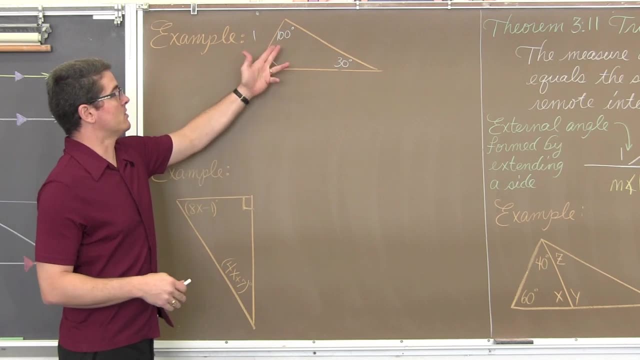 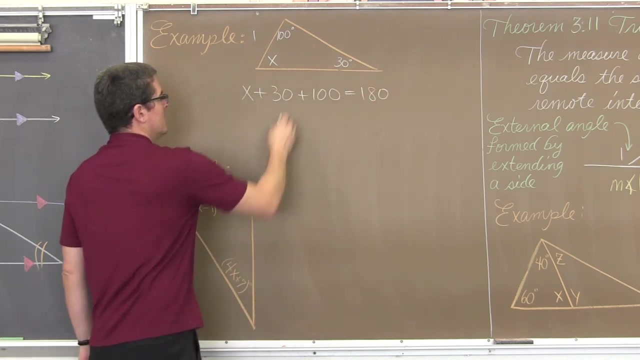 up to you to just memorize that fact. The interior angles of any triangle always adds up to 180 degrees. So if we know that these three angles must add up to 180 degrees, that is how we are going to solve the problem. or solve for x: Make them add up to 180 degrees. You can keep. 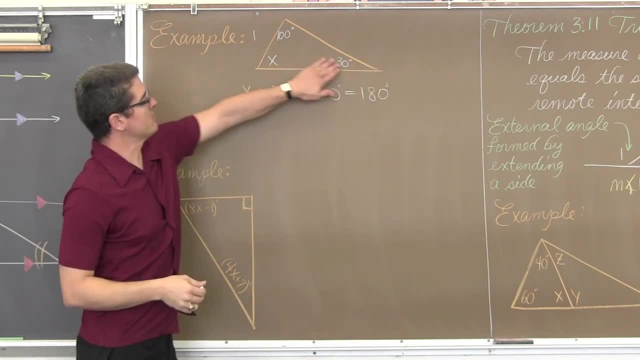 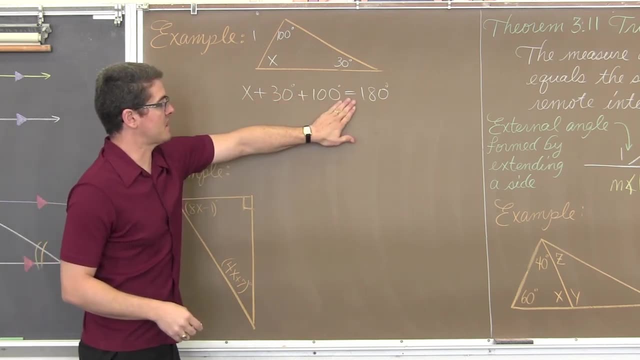 the degree marks in here, since we are looking at the entire measurement of these angles. We have like terms on the left side of our equation. These three terms are on the left side of the equal sign, So we are going to combine like terms. 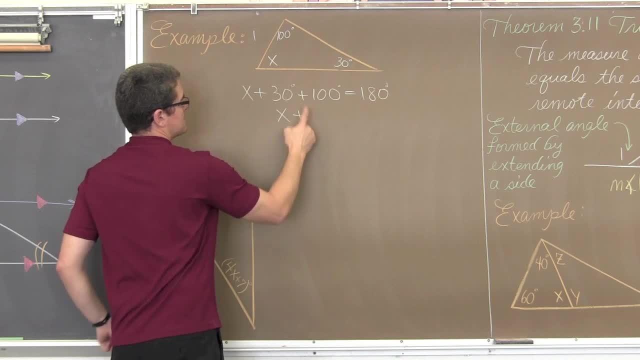 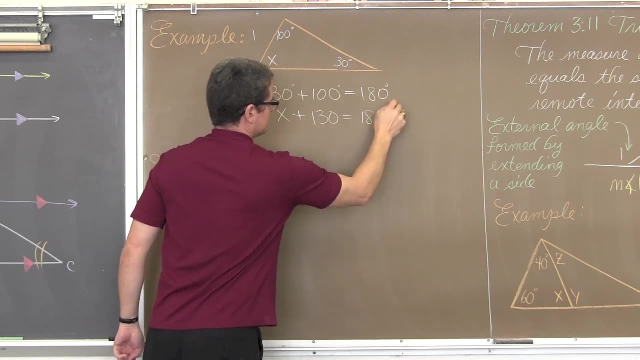 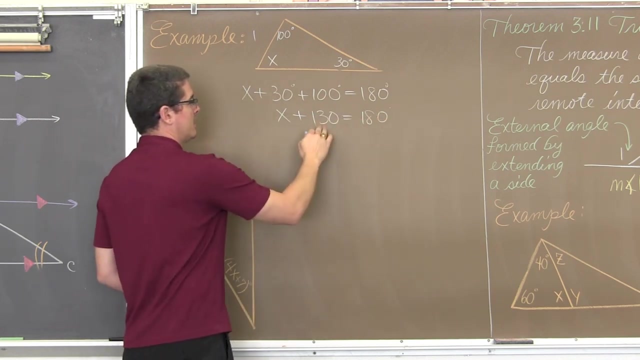 So x is equal to. excuse me, x plus 30 plus 100 is 130.. equals 180 degrees, Or just 180.. We need to get the 130 away from the x and to the other side of the equation Again, any time you want to take a number from one side of an equation over to the other. 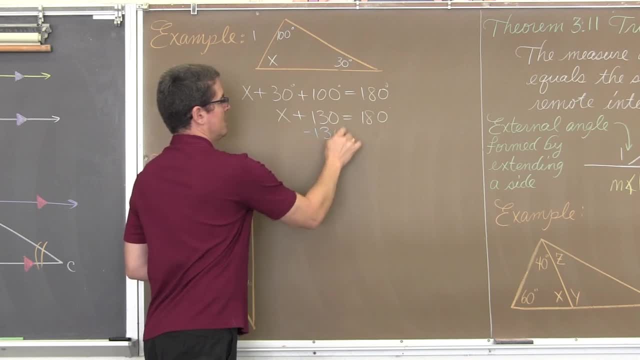 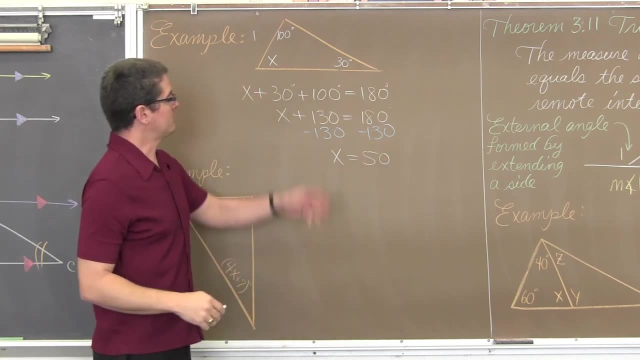 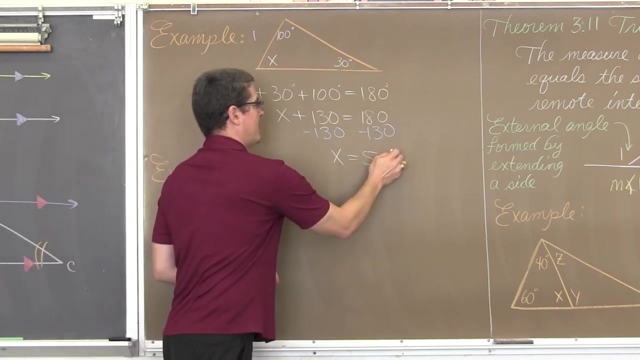 you must do the opposite math operation. We are going to subtract both sides by 130.. That is going to give us: x is equal to Now. if x was part of a larger expression, like it will be down here, I would not put a degree mark on it. but x is the entire value of this angle. so let's go ahead and call. 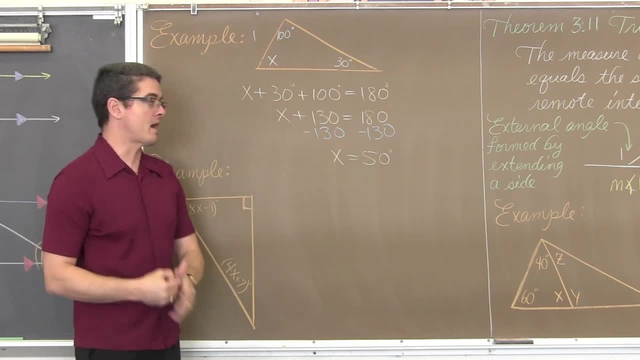 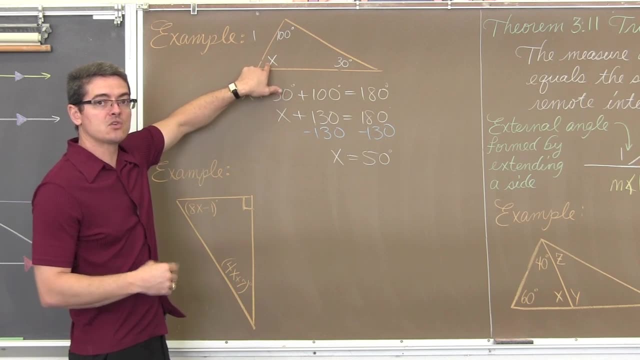 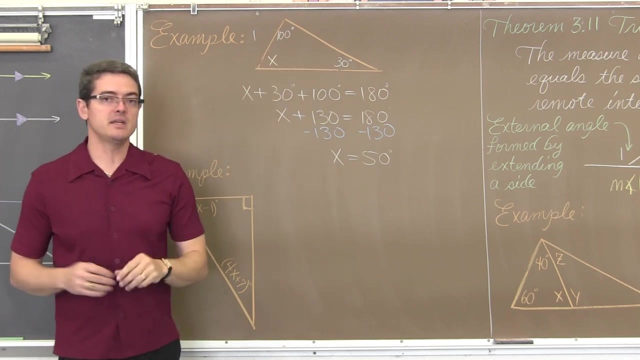 that 50 degrees. If I want to make sure that my work is right- I have not made any algebraic mistakes- then I would take this 50 and plug it back into the triangle, or take the value of x and plug it back in here and make sure that these three interior angles do indeed add up to. 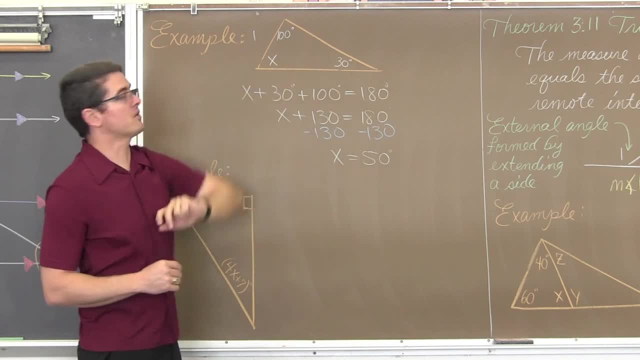 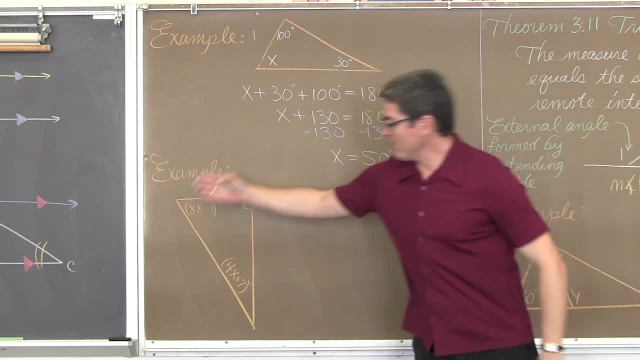 180 degrees. So we have 50, and 30 is 80, plus another 100 is of course that 180, that we set the three angles equal to Well. here we have another example. let's say right triangle, because we have a right angle. 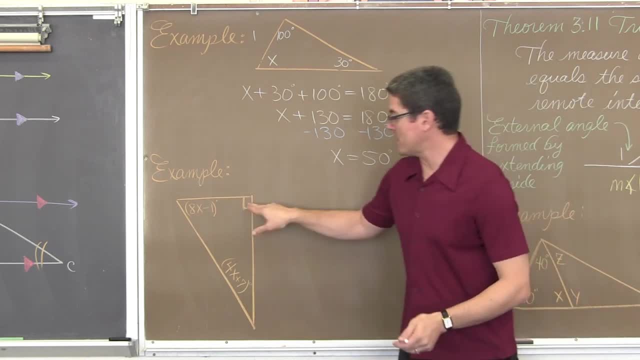 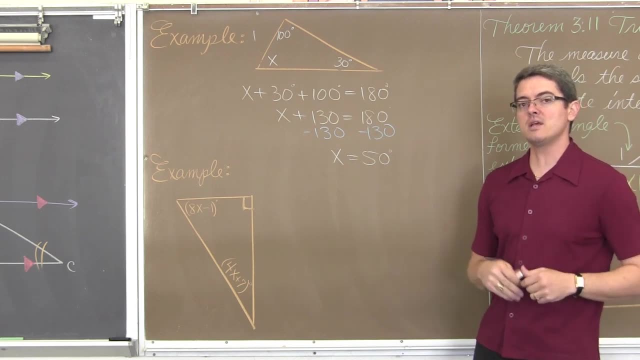 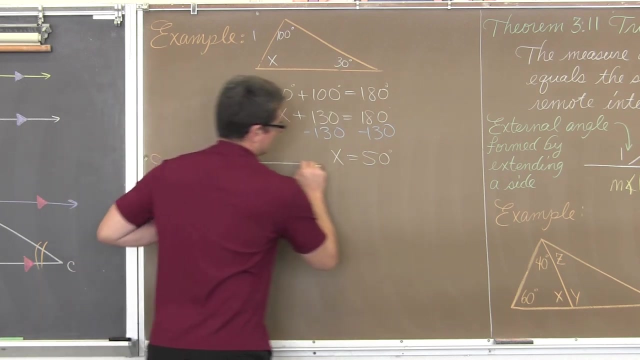 And these three angles again are all on the inside of the triangle. so they are the interior angles And the sum of the interior angles of any triangle It is always again 180 degrees. So we are going to do 8x minus 1, let's draw a division line there: 8x minus 1, plus 4x. 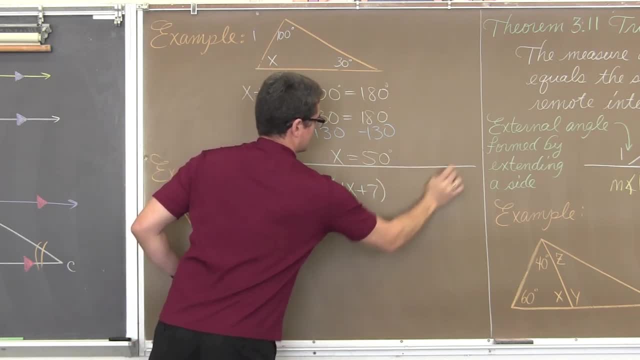 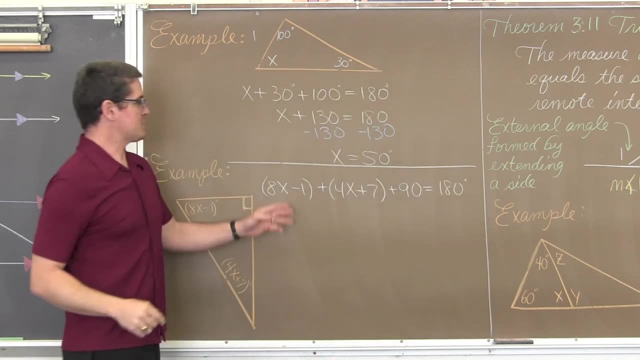 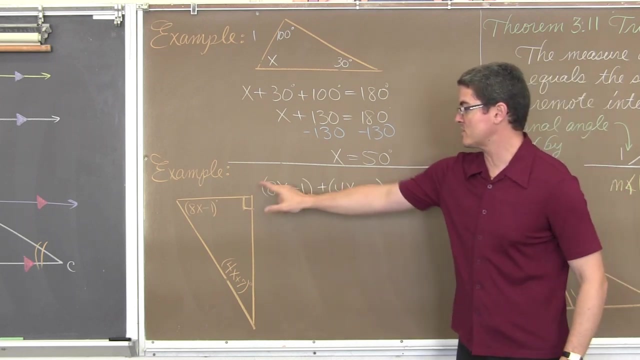 plus 7, and that is equal to whoops. I forgot my 90 degree angle here. my right angle plus 90 is equal to 180 degrees. These parenthesis- I am only putting these parenthesis There to highlight the angles. they are not really going to do anything. there is no coefficients. 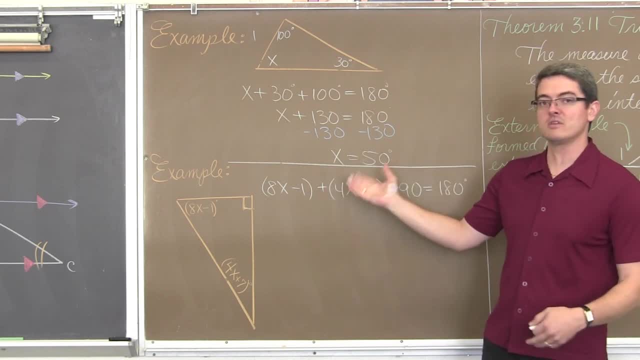 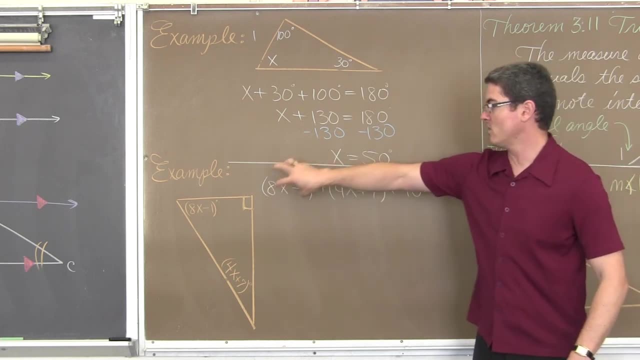 out front. If that were a minus sign it would have to be distributed, but it is just a plus sign. So there is no coefficients out front, there is no exponents, there is no fraction bars. I am just highlighting that I have taken the one, the two and the three angles that are 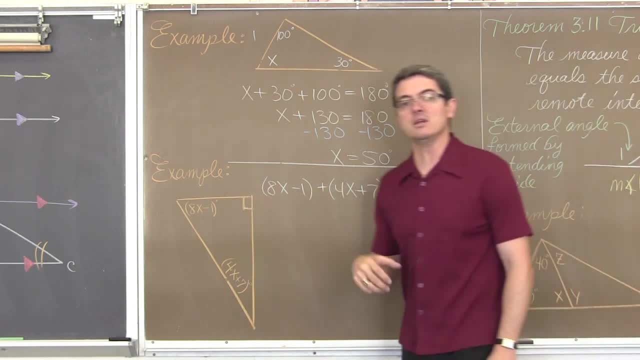 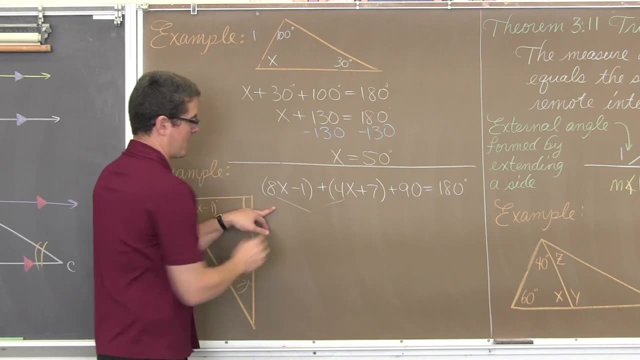 inside of the triangle. and I am making them add up to 180 degrees, The sum of the interior angles of a triangle. So I have got some algebra again to deal with. So what do I have? I have got 8x and 4x. 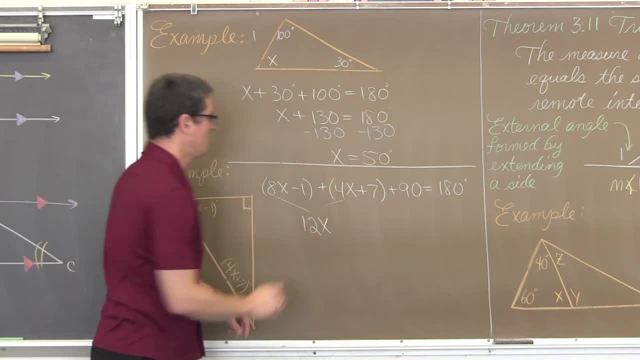 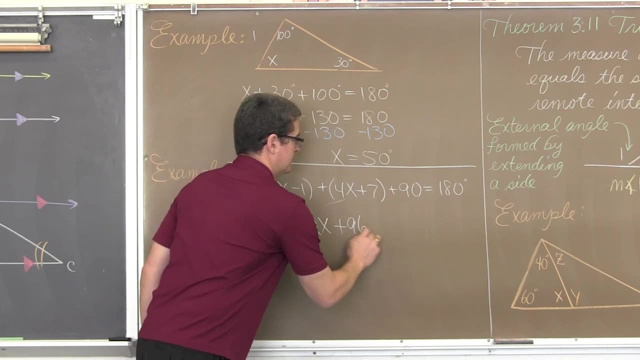 Well, 8 and 4 make 12.. We have negative: 1 plus 7 is 6.. And now we have 6 and 90 is 96.. Equals 180.. Again, we are trying to solve for x, so we are going to subtract both sides by 96.. 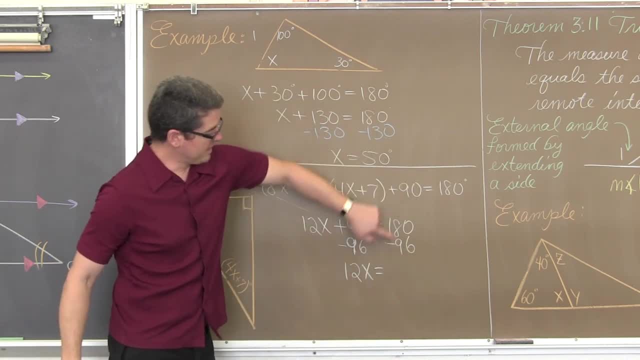 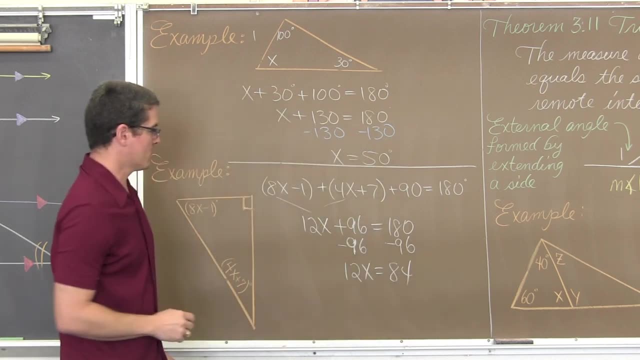 And we have: 12x is equal to 180 minus 90 is 90. And 90 minus 6 is 84. And then we are going to divide both sides by 12 and get x is equal to. let's see here: 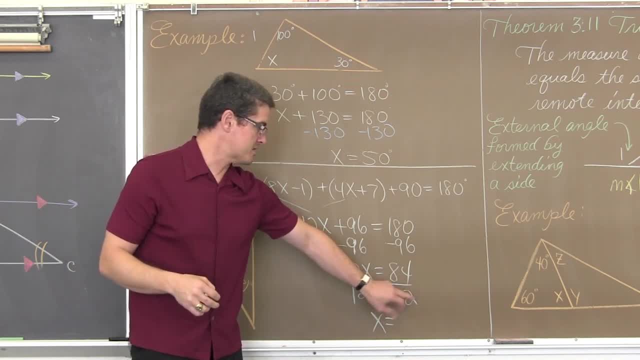 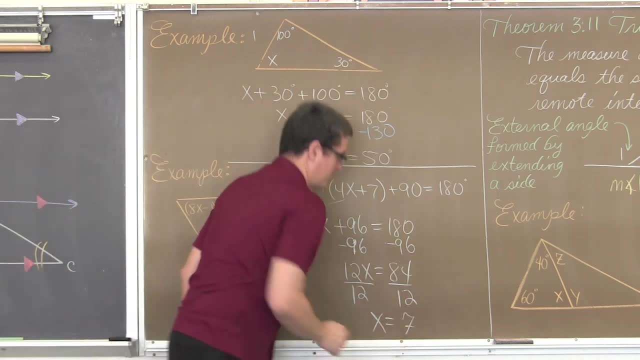 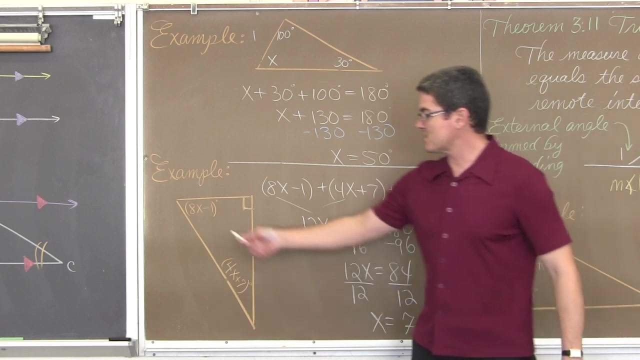 10 times 7 is 70, and 7 times 2 is 14,. 70 and 14 makes 84. So 84 divided by 12 is equal to 7.. So that should be the right answer. If we want to make sure that it is the right answer, then we would take the 7 and plug. 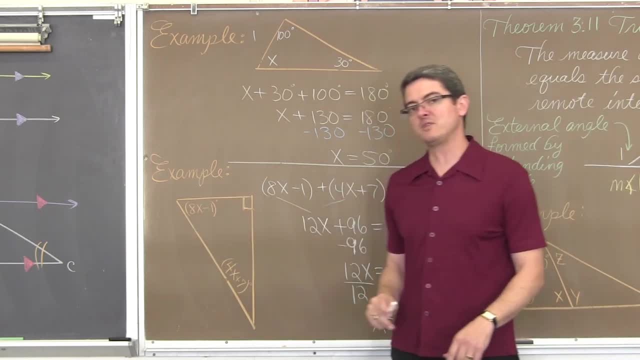 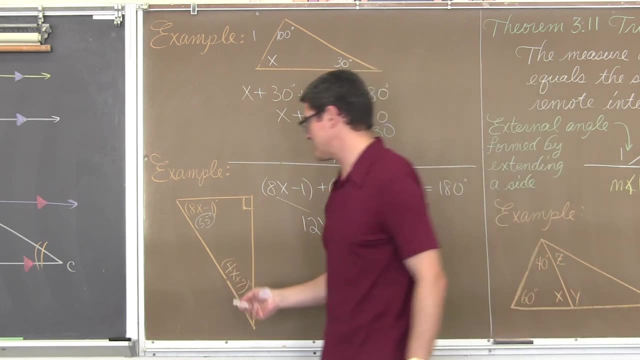 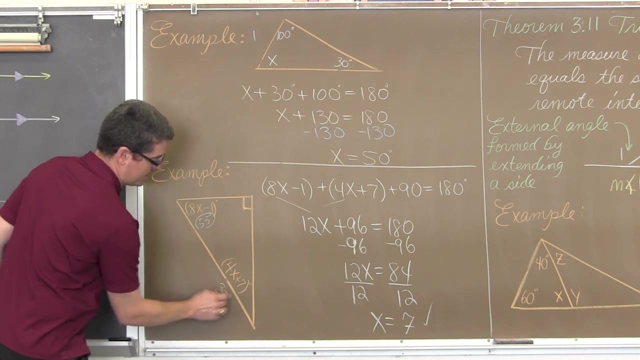 it back in here And let's see here: 8 times 7 is 56,. 56 minus 1 is 55 degrees. We have again the 7 here: 4 times 7 is 28,, and 28 plus 7 is 35 degrees. 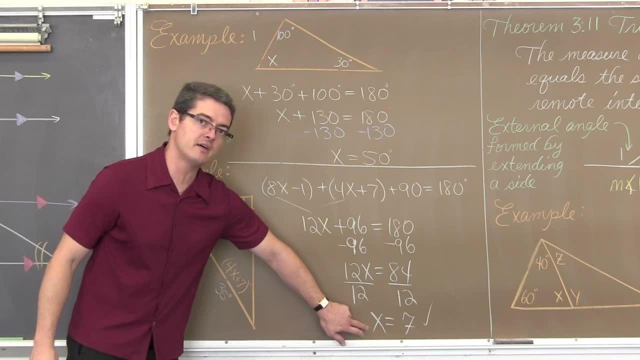 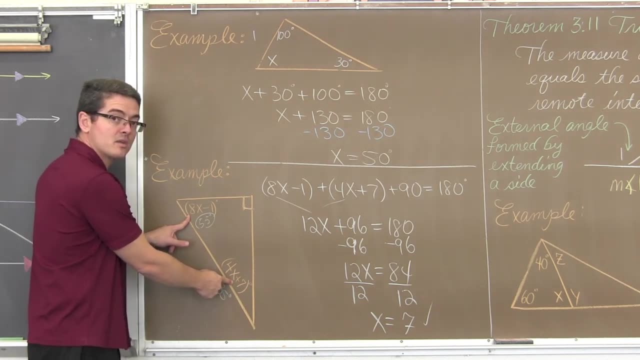 If you are not catching on what I am doing, I am taking this value of 7 that I think x is equal to, and I am plugging it back into my expressions that are supposed to be the size or the measure of these angles. 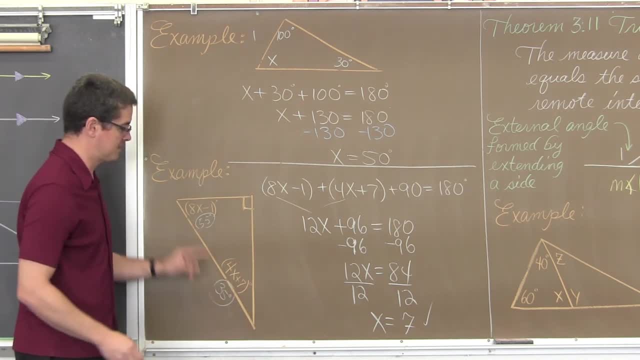 And 55 plus 35 adds up to 90,. 55 and 30 is 85, and then another 5 is 90. And these two together with 90 make a 90 degrees along with a 90 degree angle. Again, that does add up to 180. 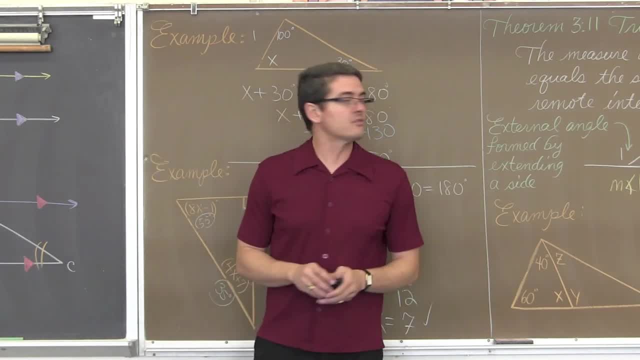 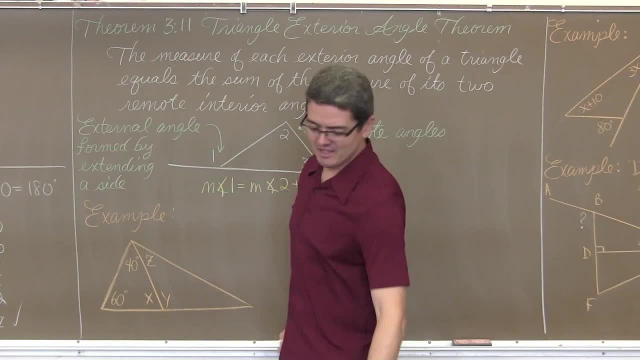 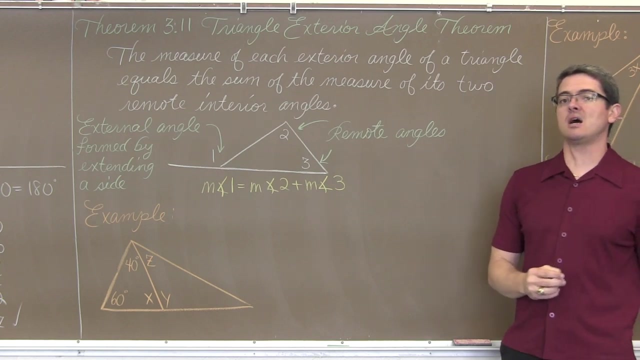 So it looks like I have done my work right. We have one more theorem and three examples to go along with that. Be right back. Theorem 3.11.. Triangle- Exterior Angle Theorem. The measure of each exterior angle of a triangle equals the sum. that means you add them up. 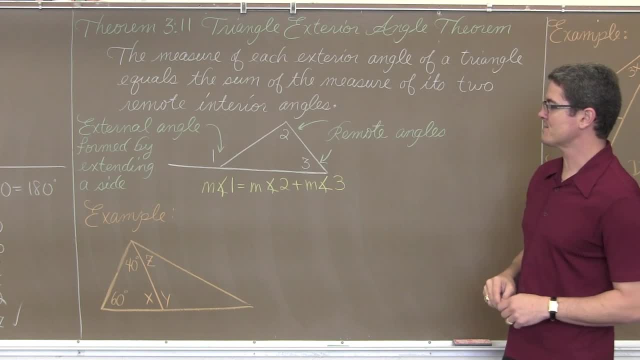 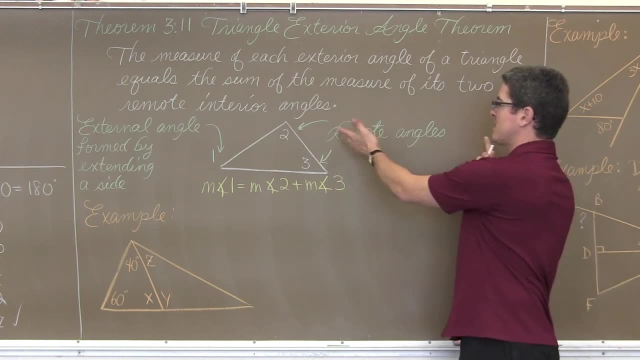 of the measure of its two remote interior angles. Now this is a triangle. We have two interior angles marked. They are going to be set up and called the remote interior angles here in a second. So I left off the word remote, excuse me. the remote interior angles. 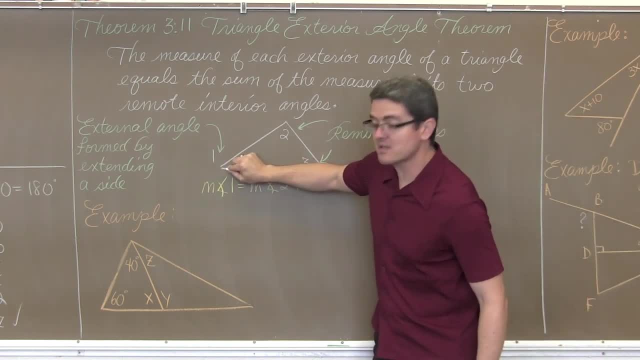 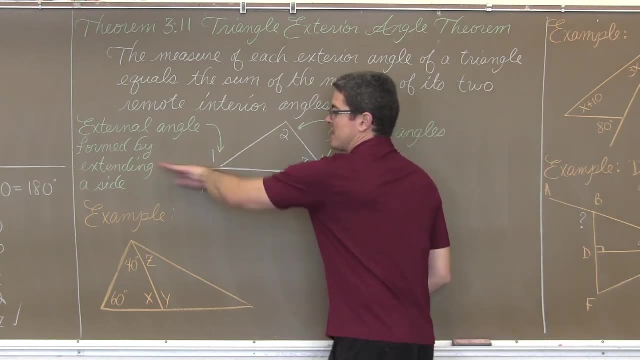 And we are going to make the exterior angle by just taking one of the sides of this triangle and extending it straight out, Not bending it. It is not like a. it has to be a line. You are extending the line beyond the vertex of that triangle. 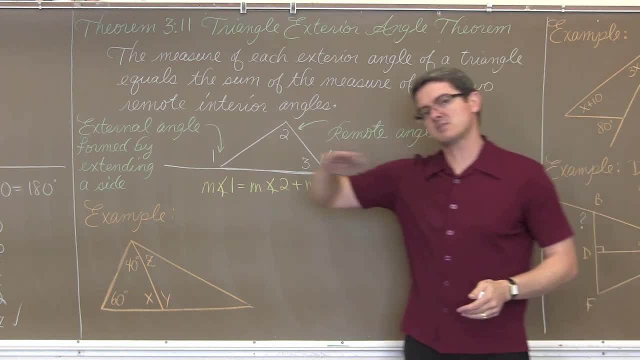 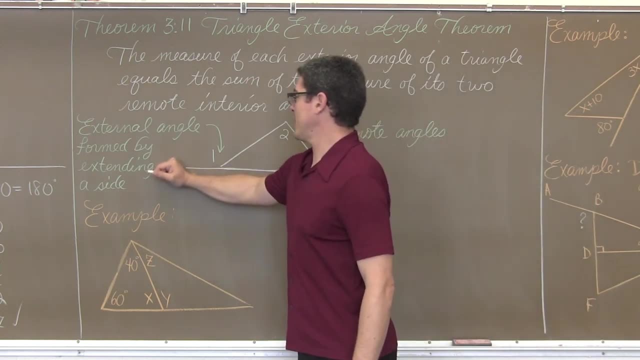 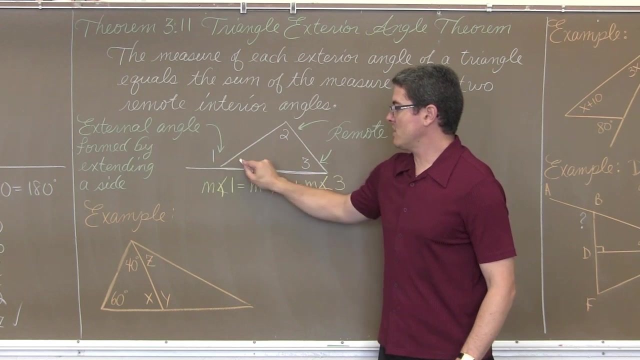 Or indeed, if you take any polygon, just a straight sided figure, and extend one of the sides beyond one of the vertexes, you create an exterior angle. So this exterior angle, angle 1, that we have it marked off as well, the interior angle. 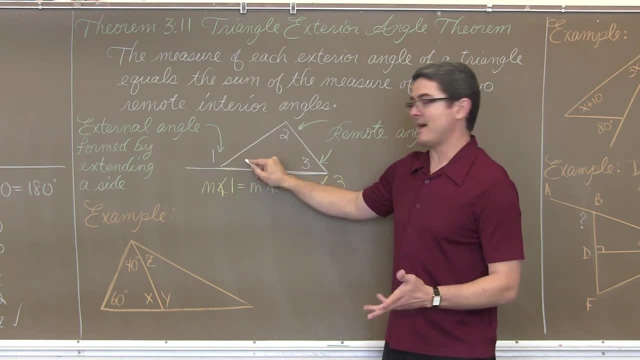 that is adjacent to this exterior angle, The interior angle that is adjacent to this exterior angle. The exterior angle is just that, it is just an interior angle. When we talk about the remote interior angles, we are talking about the two angles in the 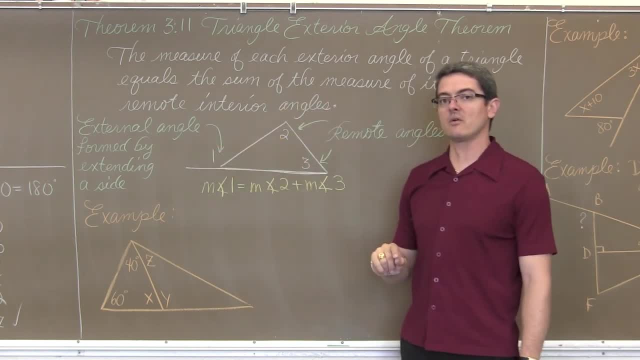 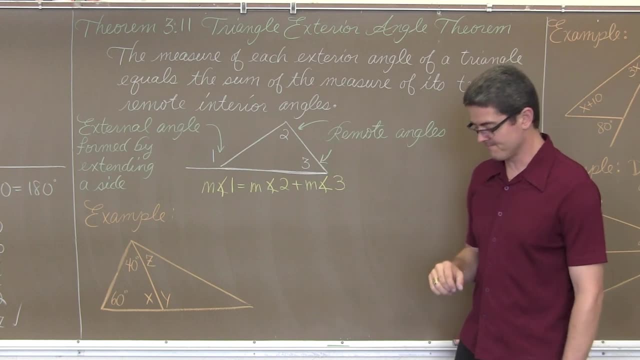 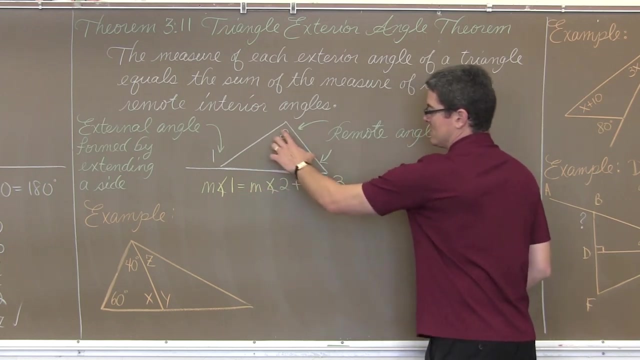 triangle that are not adjacent to the exterior angle. Remember, adjacent is you share a vertex and you share a side. So this is the adjacent interior angle. These are the two remote angles. Why is it that the measure of the exterior angle is equal to the measure of the two interior? 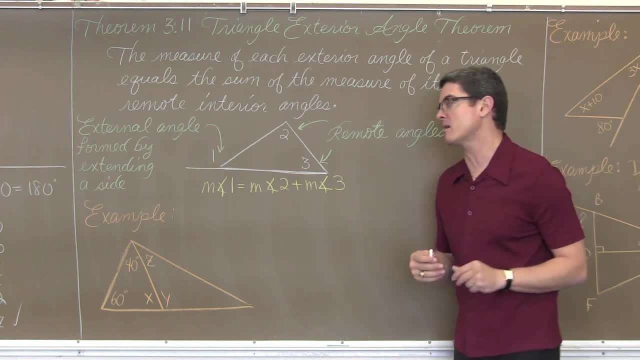 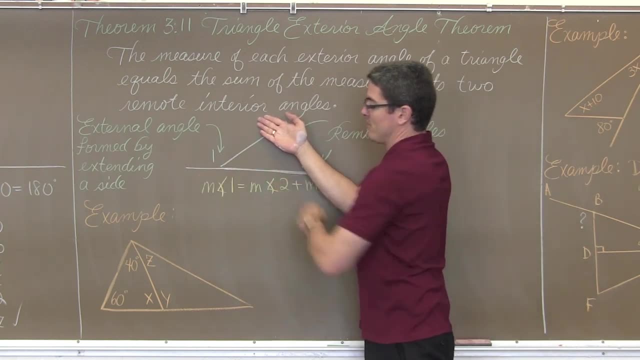 angles added. I am not going to do a two column for this either, but I do want to talk about it. But if I cover up this part of the diagram, what do you still see? You see two adjacent angles forming a straight line. 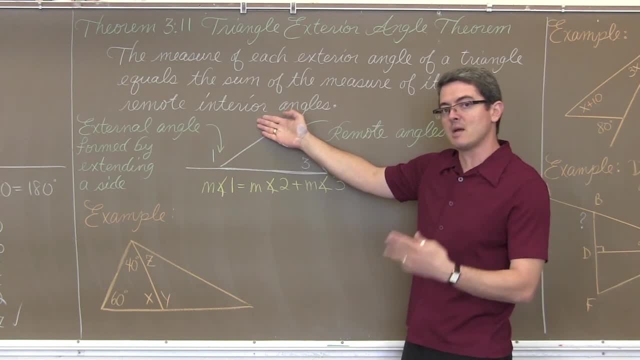 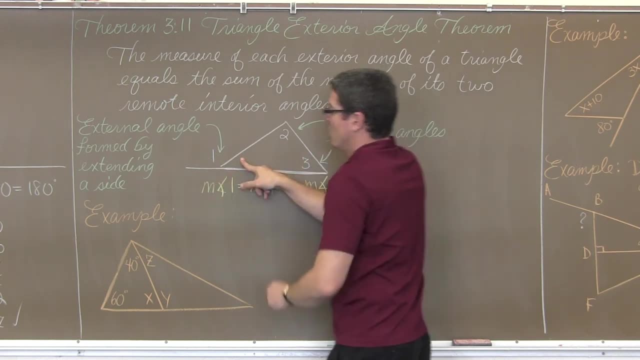 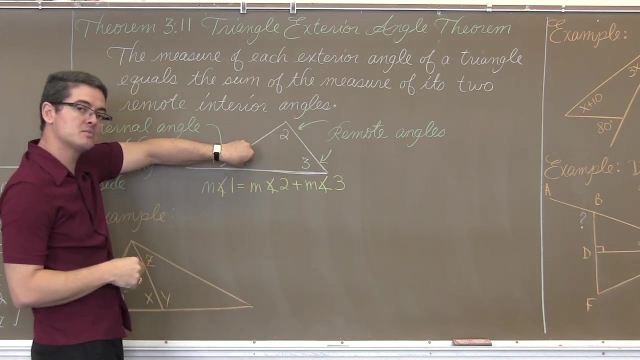 That is again. how many times has this come up? It is a linear pair, they are supplementary. This angle plus this single angle has to add up to 180 degrees. Well, this angle plus these two have to do what The inside of your triangle has to add up to 180 degrees. 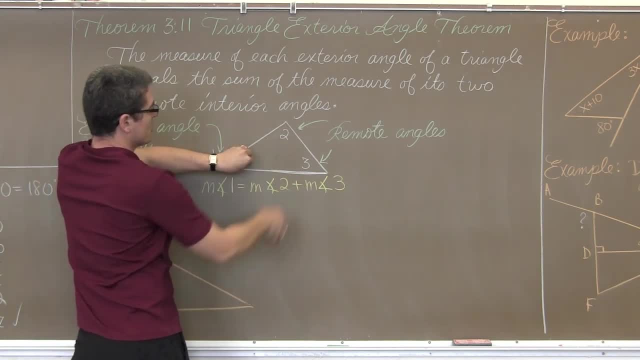 So this angle plus one adds up to 180.. This angle plus these two together have to add up to 180 degrees. So if this is 30 degrees, here this has to be 150.. If this is 30 degrees, here these two have to equal 150. 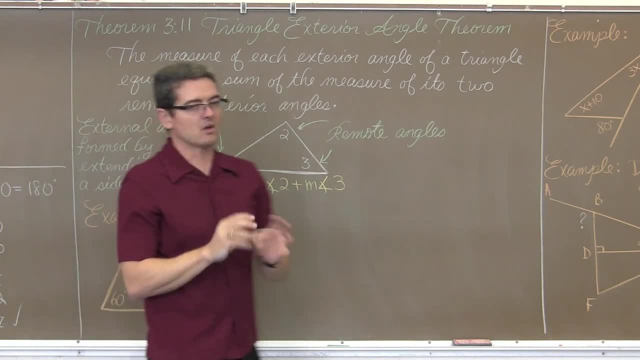 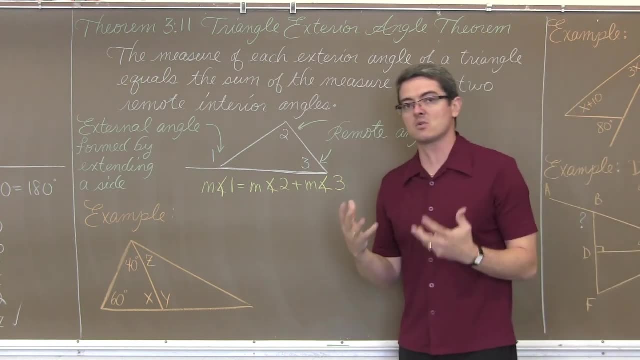 So it adds up to 180.. So that is sort of a super quick. it is not really proof, because I did not make each statement and talk about the reason behind each statement, but that is what is going on there And that is why your exterior angle equals 180.. 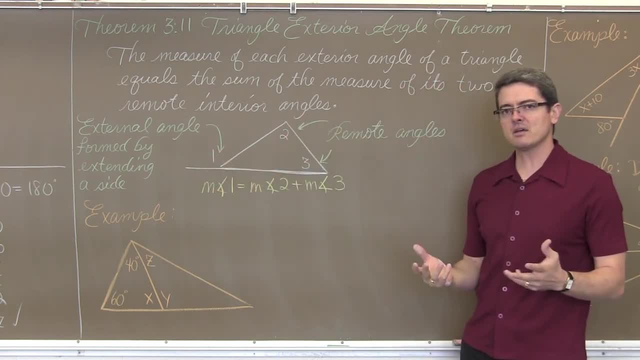 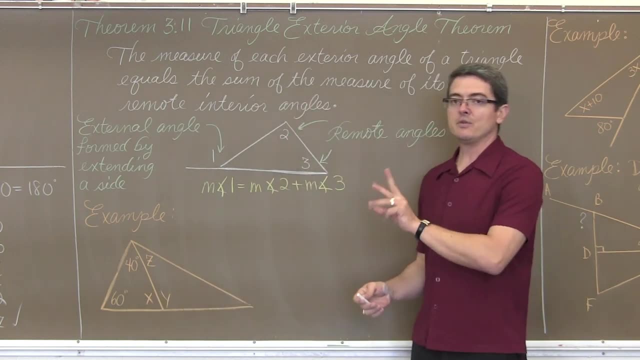 It is an angle that is equal to the sum of the two interior angles. So how is that going to work? Well, I have got an example here. we are going to do three of them. This is going to combine the two theorems we just talked about. 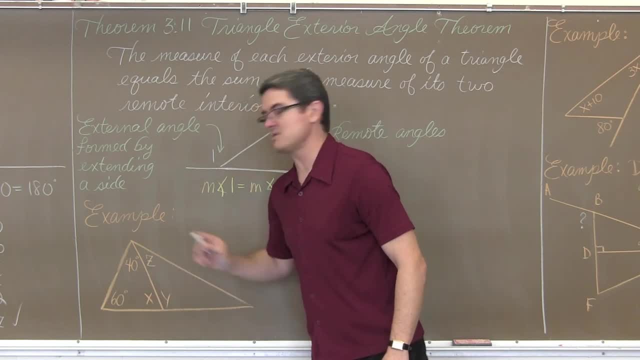 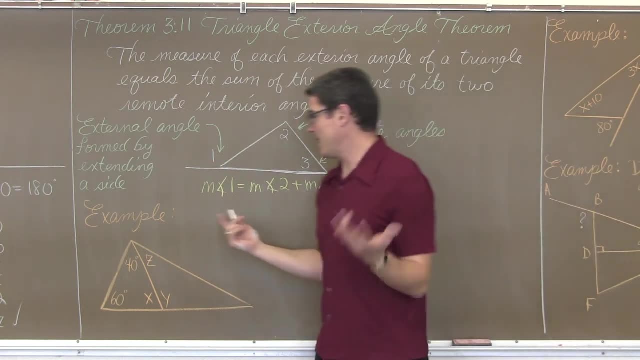 We are going to find out what x, y and z are equal to, And you kind of have to go in a certain order. I cannot look at this right now and immediately tell you what z is, And I am not going to be able to finish the problem at all if I do not tell you that this. 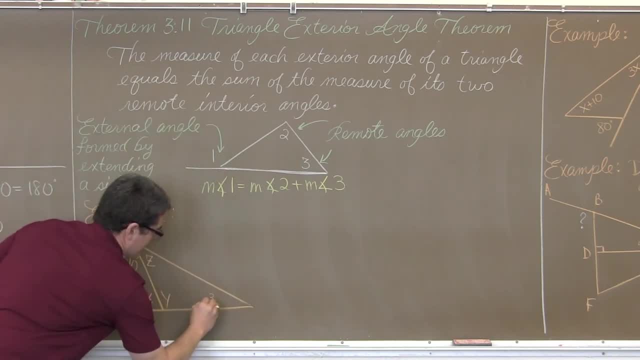 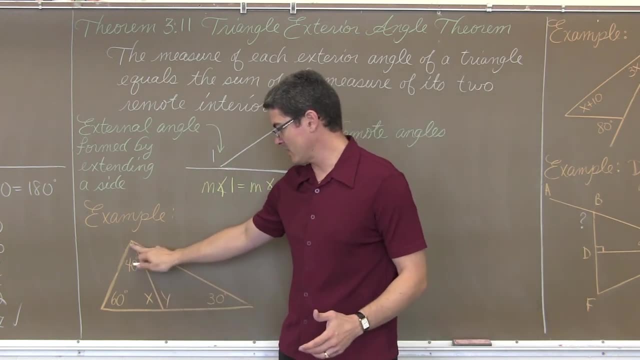 angle right here is: 20 degrees is equal to 30 degrees. That is one of the numbers. Ok, So let's find out what x is equal to. I am looking at this triangle right here. You are probably not going to see this different. 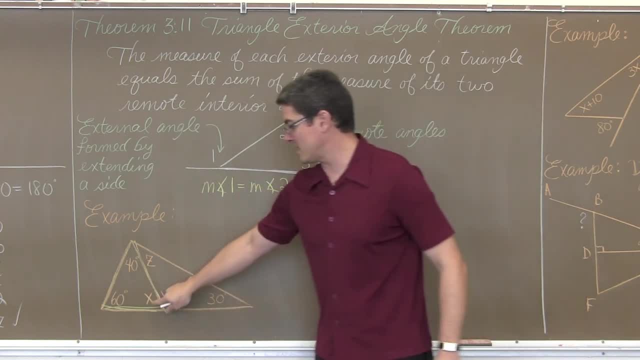 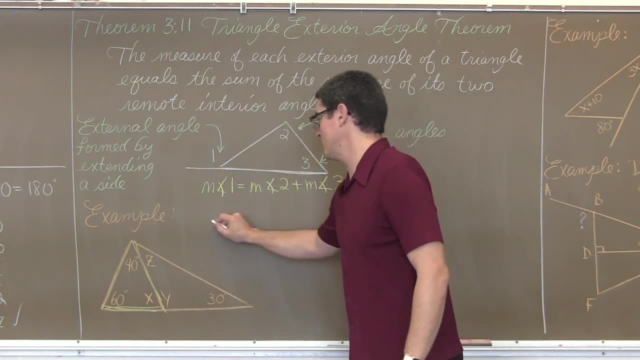 color on the camera. But this triangle right here, x is in the interior of this triangle and I have two of the angles already and I only have one left. So if I want to find out what x is equal to, I just do: 60 plus 40 plus x is equal to 180.. 60 and 40 makes 100. And 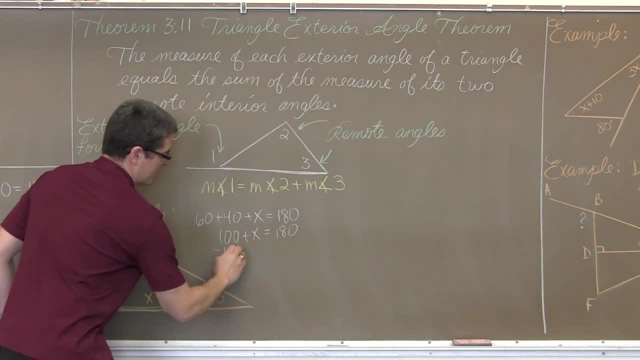 if I bring this 100 from the left over to the right, with subtraction you always move from one side to the other with an opposite math operation and this 100 is not multiplied or anything, It is just its own term. so we subtract it, We get: x is equal to 80.. Now 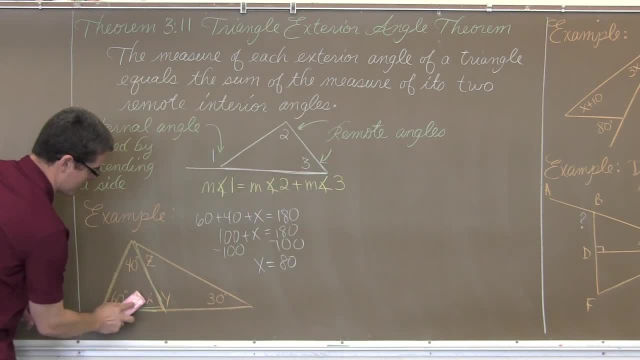 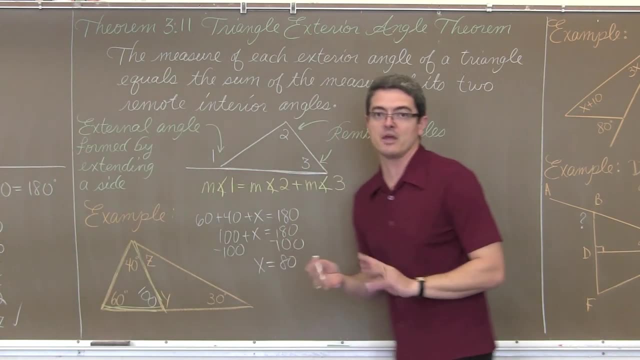 that I have got this equation, I am going to go to the next one. Let's see what this. Now that I know what x is equal to, I am going to go ahead and erase that in my diagram and put 100 there. So I remember what it is and I see it is relational a little bit easier with all the. 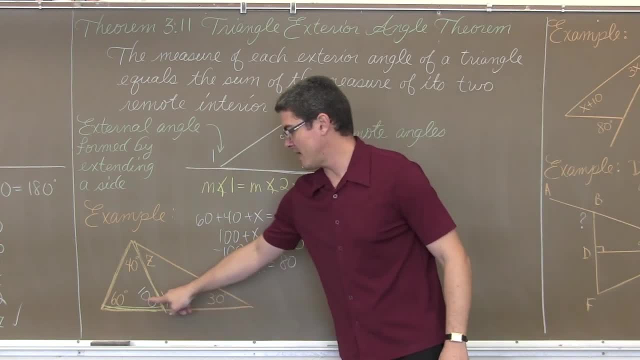 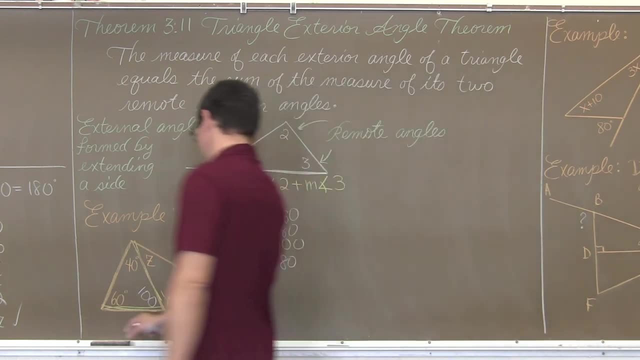 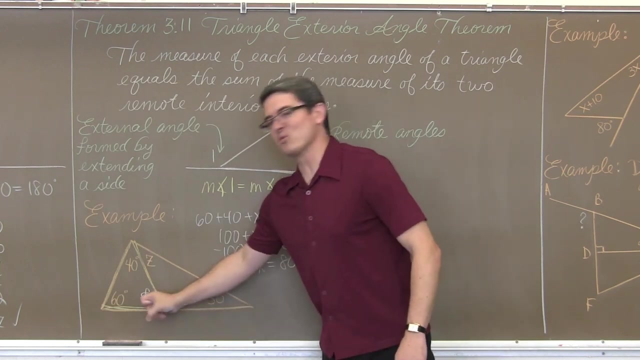 other angles. Well, when I see 100 degrees here, I am looking at 100 degrees here, so this is certainly um, that would be 80.. let's try that again. When I see 80 degrees here and I see the y next to it, this is a linear pair. 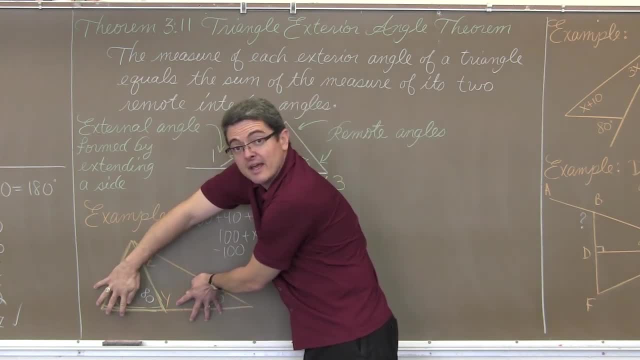 There's a lot going on in this diagram, but I am looking specifically at angle y right now, and angle y is adjacent to the angle now. that is marked as 80 degrees and they are forming a straight line. These are a linear pair, So a linear pair must add up to 180 degrees. 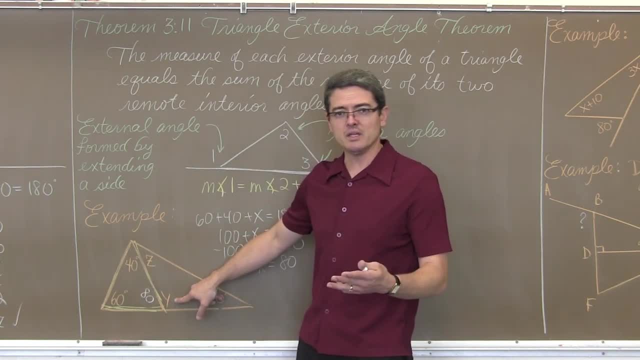 So y is equal to well, it is going to be 100, and I can justify what y is based on the fact that these are a linear pair. But I can also justify what y is because, if I cover up this part of the diagram, what? 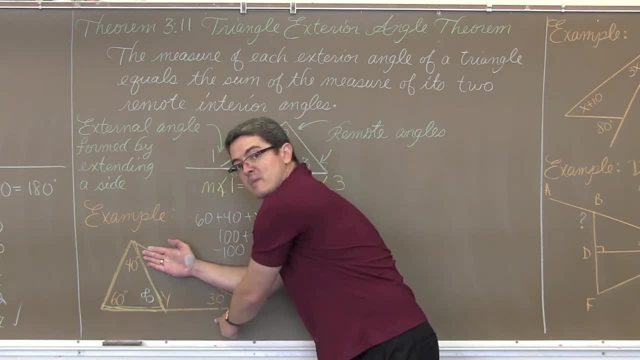 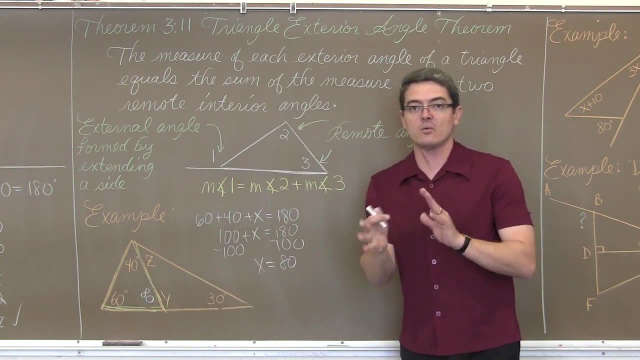 do I have. I have a side of this triangle just extending out into space. This is an exterior angle and it is equal to the sum of the two remote interior angles. So either way you look at it, whether it is a linear pair and it is 180 minus 80 is 100,. 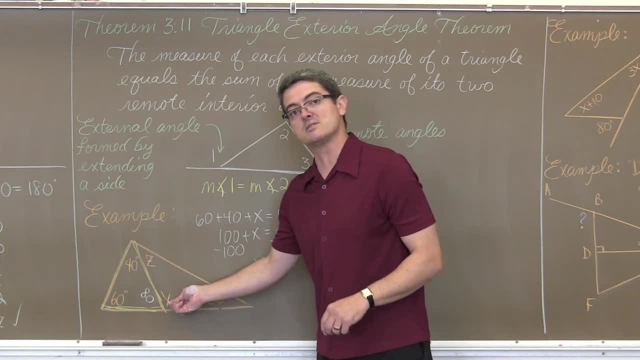 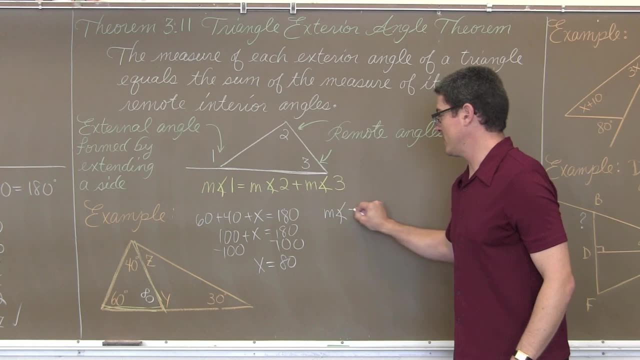 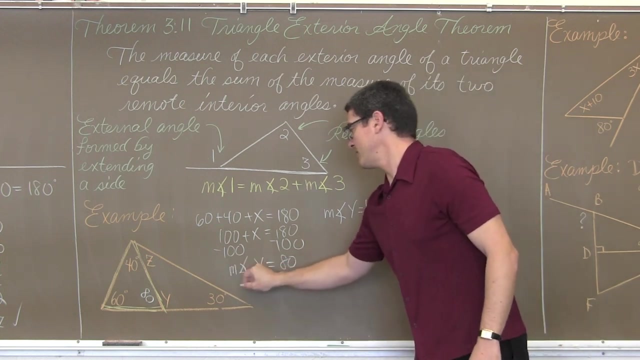 or whether this remote external angle- excuse me- is the sum or equals the sum of my two remote interior angles. the measure of angle y is going to be equal to 100. And this was the measure of angle x. I should have had that measure of angle x in this notation as well. 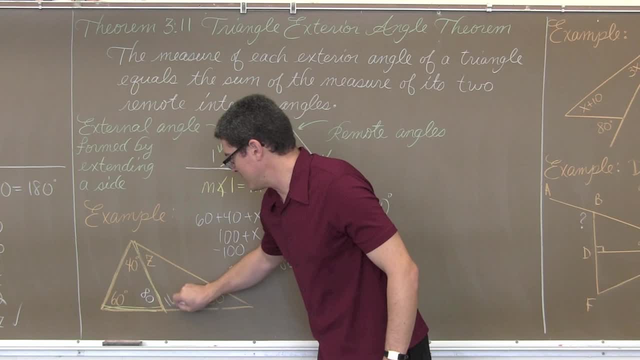 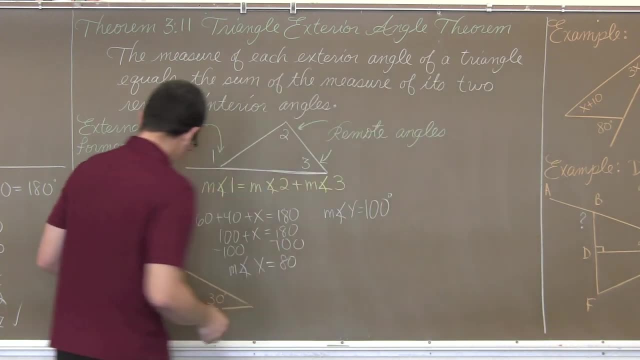 So now I know that y is 100 degrees. that's probably why I wrote 100 there. I was thinking of the answer, and now I want to find out what angle z is. Well, now Let's just take this diagram out of here. 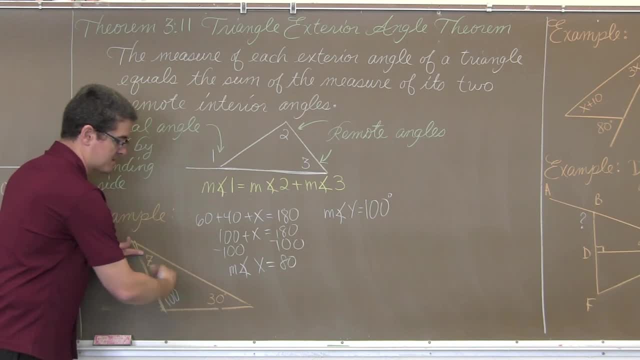 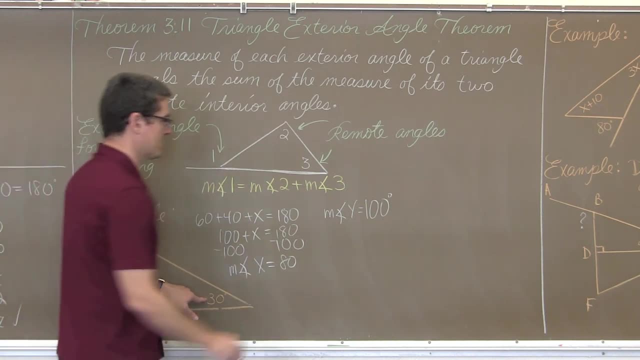 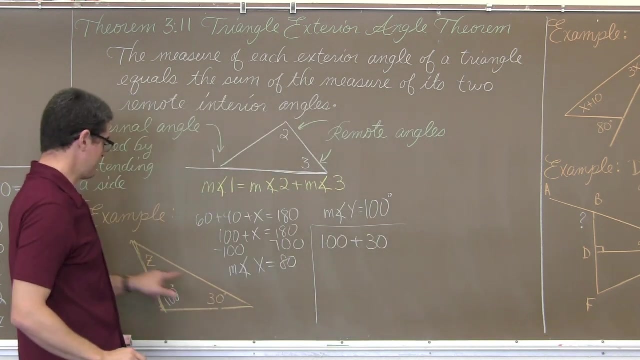 You know, z is part of this triangle that was on the right hand side of my diagram. I know two interior angles. I only have one left, So 100 plus 30, see, let's put this here: 100 plus 30, plus the measure of angle z. 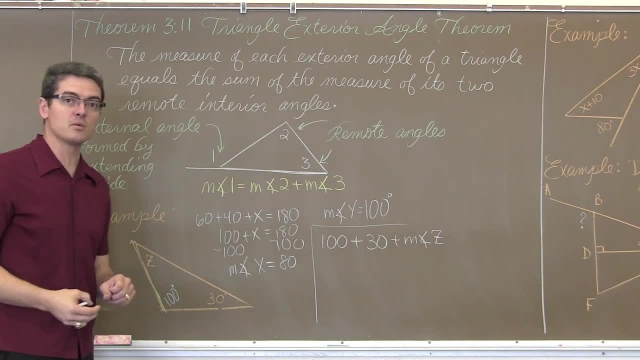 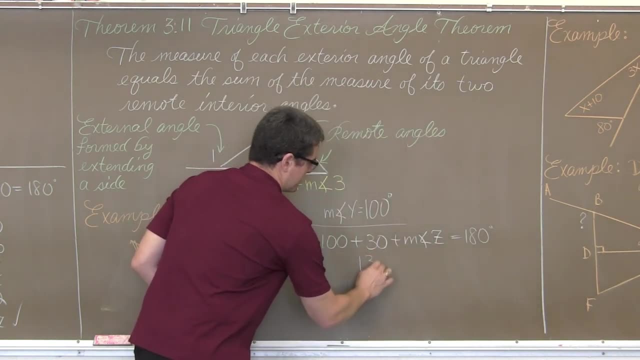 Or you could just put z. I am sure your teacher would be happy with that as well. just knowing that you are working with this variable That has to add up to 180 degrees, 130 makes 130.. We subtract both sides by 130.. 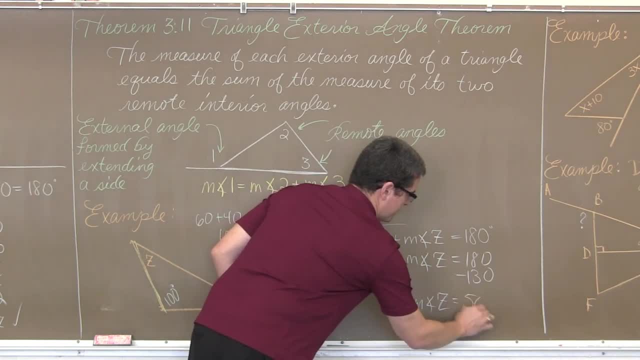 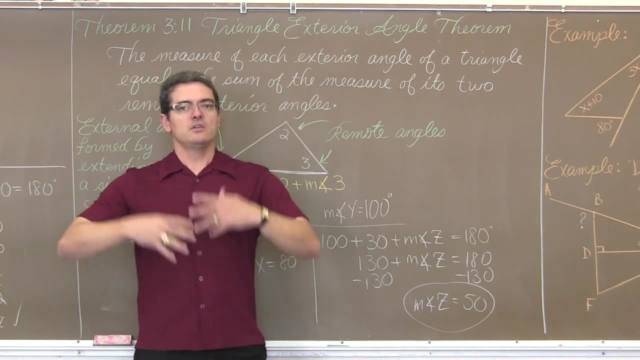 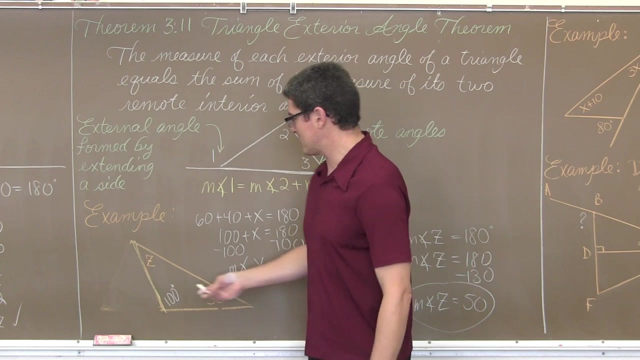 And the measure of angle z is equal to 50.. Maybe I might even want to caution you to use the notation that your teacher is happy with I am using. I threw in the measure of angle because I just had a simple variable, a single variable. 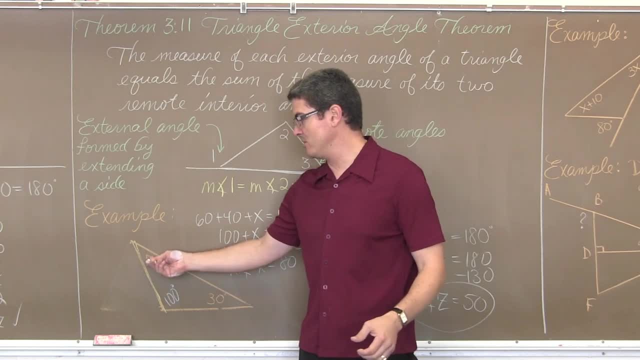 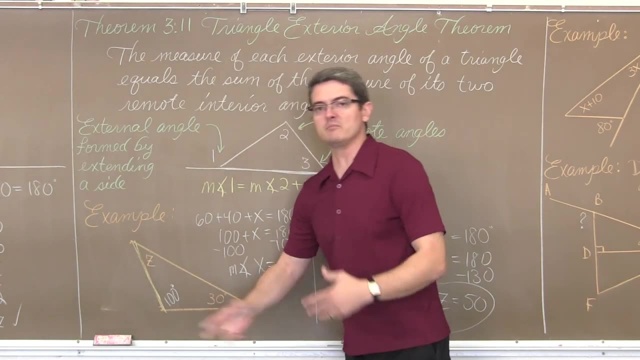 in the angle. If that were, say, 2z minus 4, probably would be very confusing to include that measure of an angle. The variable wouldn't be the measure of the entire angle. So use the appropriate notation your teacher is going to be happy with. 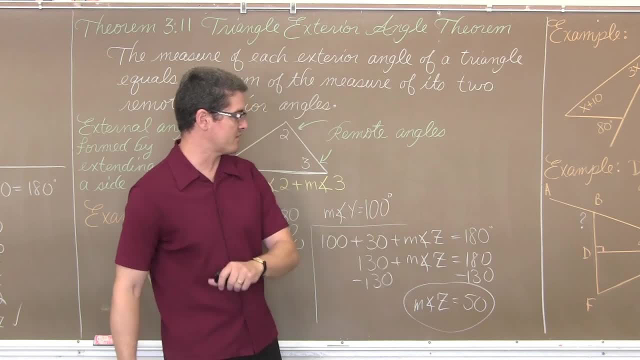 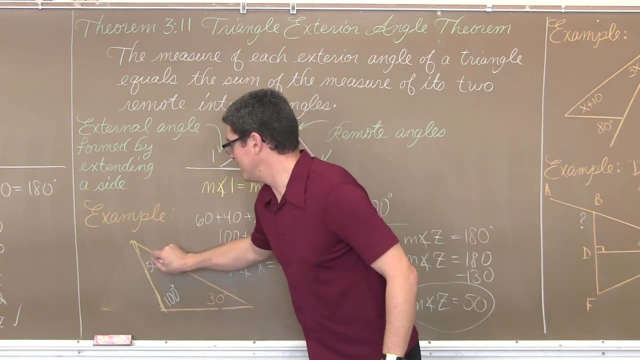 But we had a single variable there, so it would be great just using the measure of angle z or just keep the z in there, But at any rate It is 50 degrees, so 50 is there and of course I erased part of my diagram, but I hope it. 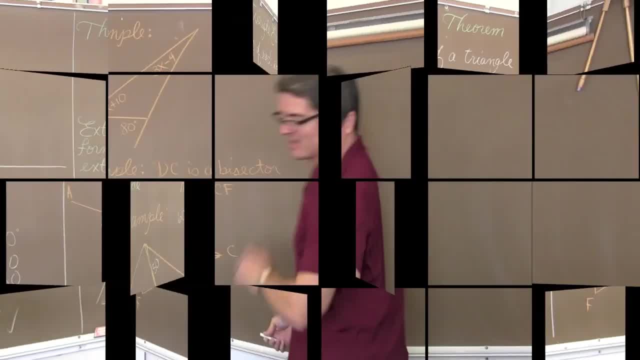 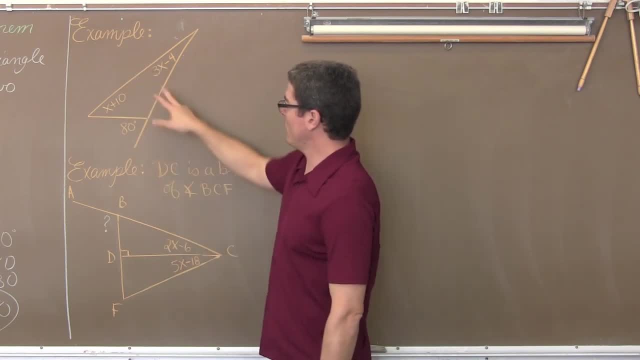 all made sense. Let's do our next two examples: BAM. Here are the last two examples. We have a triangle with an exterior angle extended and I want to solve for x. Now how am I going to do that? Well, I want to use the information the way it says. 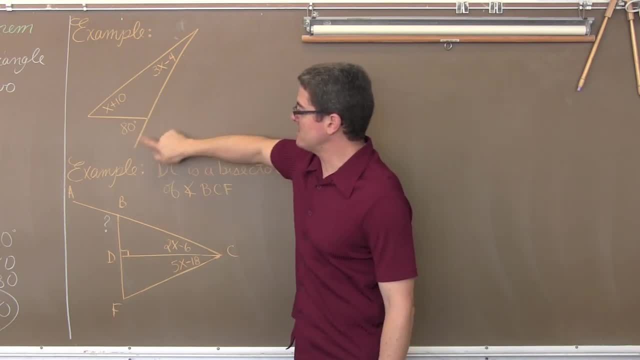 Yes, I could. knowing that this is 80 degrees and seeing the straight line, and knowing that these are linear pairs, this angle inside is going to be 100 degrees, So I could. knowing that the sum of my interior angles will always add up to 180,, I could. 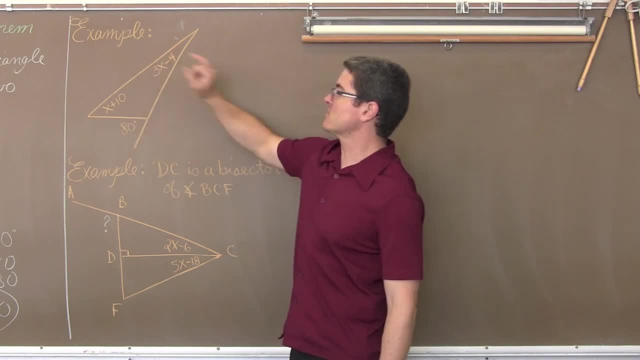 do 100 plus x plus 10 plus 3x minus 4 and set that up to equal when I add them, 180 degrees. But I also know- and it is going to be a little bit less work- that the sum of my remote interior. 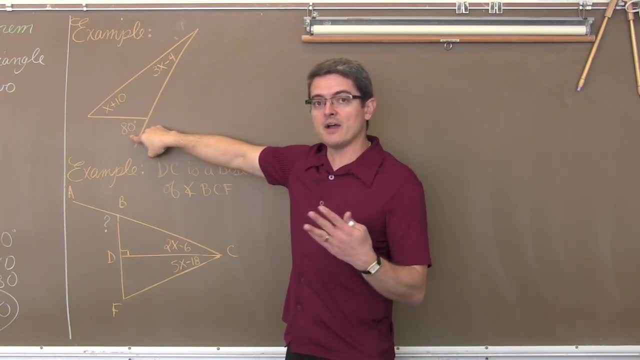 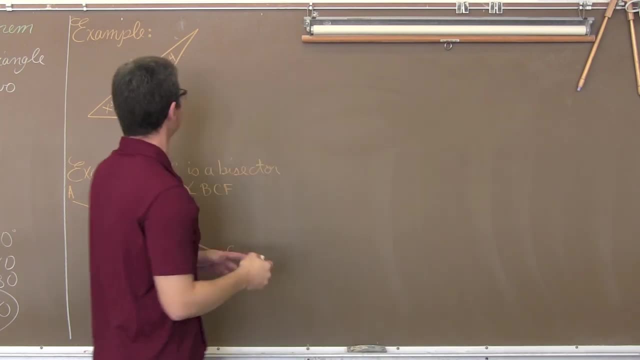 angles equals my exterior angles And if I know that, if I understand that these have to add to be equal to 80, then what I am saying is how I am going to set up my equation And again, I am going to use the parentheses just to highlight the angles that I am bringing. 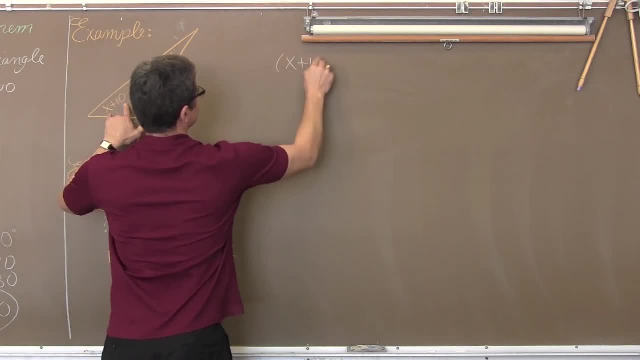 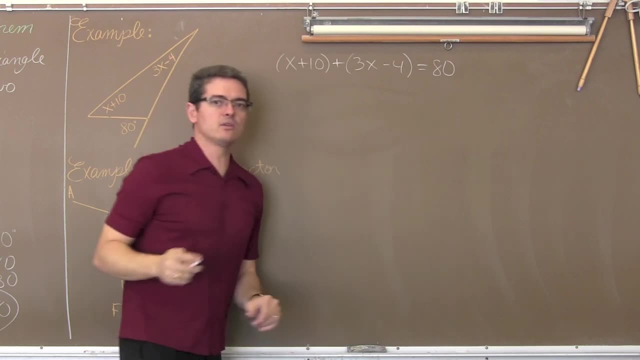 in. So we have x plus 10, so the first angle plus 3x minus 4 is equal to 80 degrees, my exterior angle. And again I just want to emphasize, we have a leading coefficient of 1.. This is just a point. 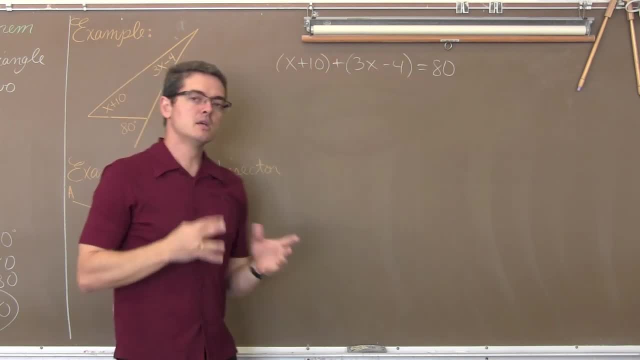 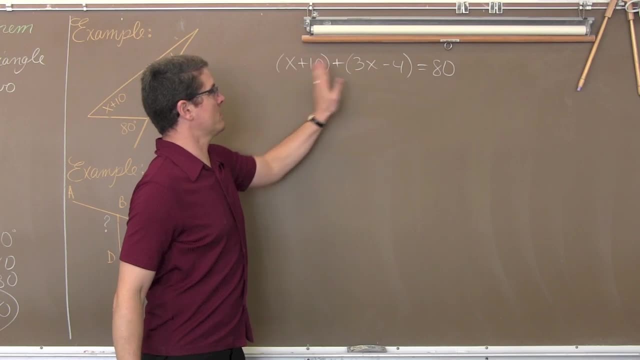 This is just a plus sign. there is no exponents, there is no fraction bars, So these parentheses really aren't doing anything. I am just trying to highlight the two angles that I am adding, the two remote interior angles that I am adding to equal. 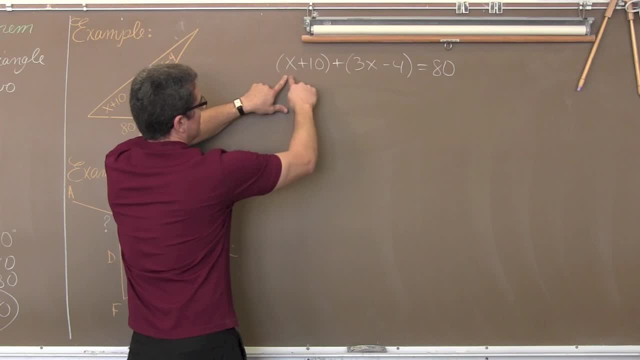 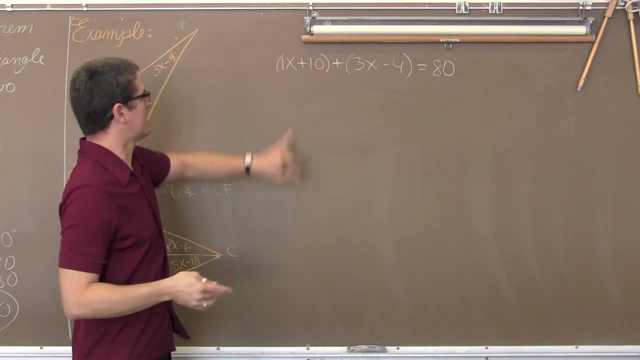 that exterior angle. So let's go ahead and add those like terms. Also, if you have a problem combining like terms, then maybe you want to go ahead and put a 1 in front of that x, so you see the number there and you remember that you have. 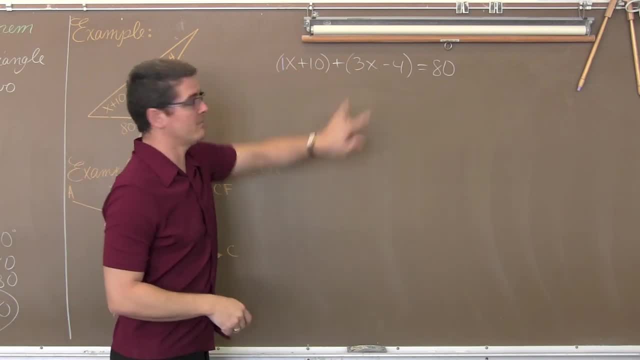 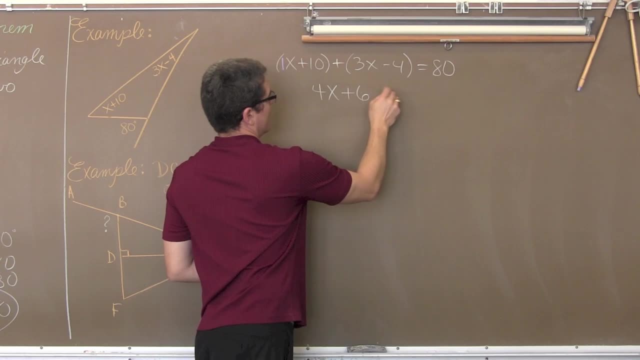 to add. So we have 1 and 3.. Well, 1 and 3 make up a lot. 1 and 3 make 4x And we have 10 minus 4, which is equal to 6. And that is equal to- I should have lined up my equal sign- equal to 80.. 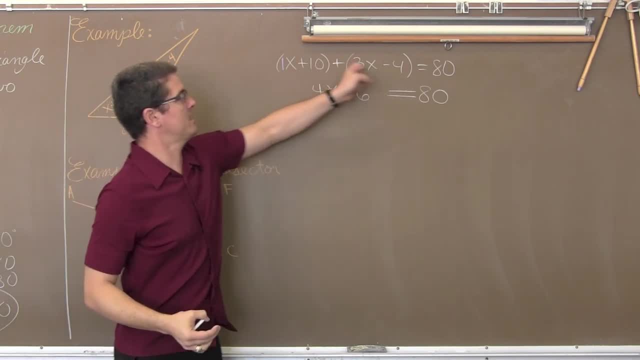 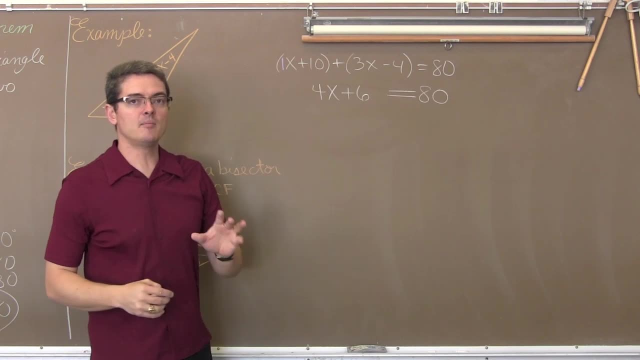 Now you will notice that I just did 1 and 3 make 4.. I just did 10 minus 4 and equal to 6.. I didn't change any signs. I didn't try to put a little plus 4 here and a plus 4 here. 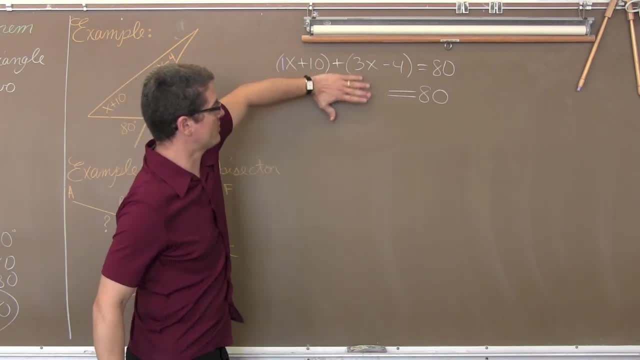 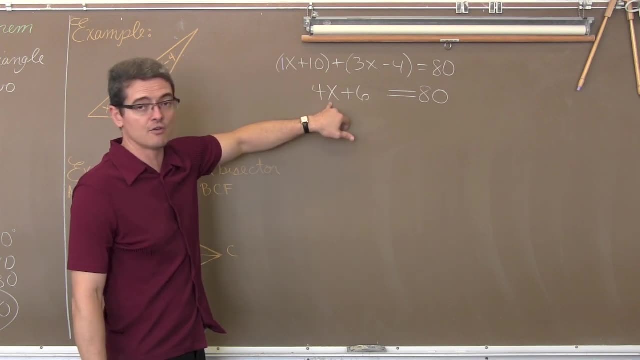 The only time you do the opposite math operation is when you are trying to move a number from one side of an equation to the other, Which I am about to do. I want to get this positive 6 away from the 4x because I am trying to solve for x. 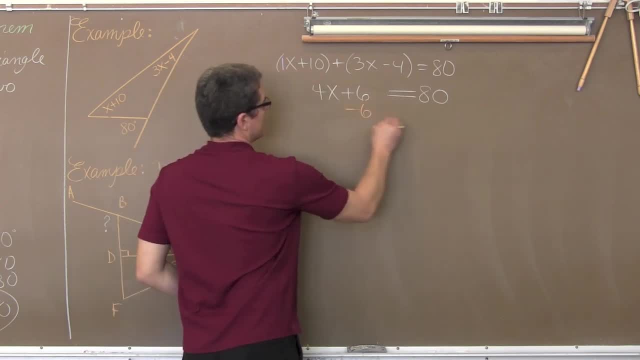 So we are going to subtract both sides by 6 and get 4x, because this is going to be 0, equals 80 minus 6 is going to be 74. And now we are going to divide both sides by 4.. 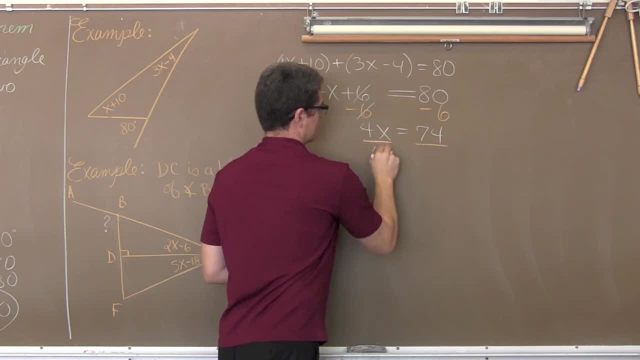 And we get x is 74.. x is equal to: am I still on the camera there? Yeah, So we have. x is equal to. let's see, this is going to be a nice round hole number. but how many 4's are in 7?? 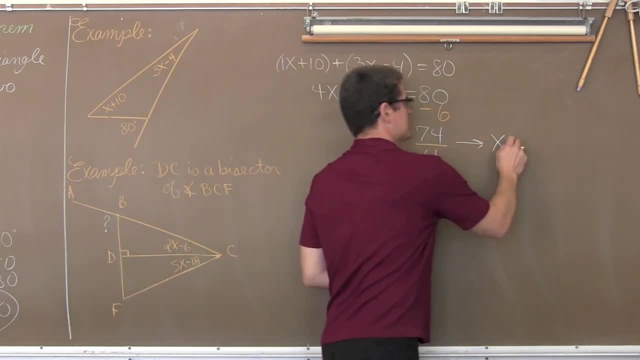 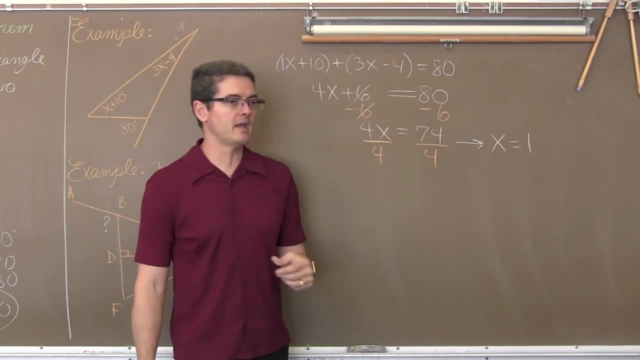 4, 8,, oh, just 1.. So it is going to be a 1, something. 4 out of 7 leaves me a 3. So we have 34.. Well, let's see here: 4 times 7 is 28.. 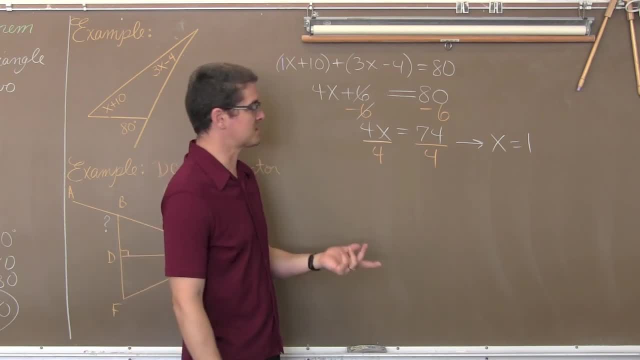 4 times 8 is 32.. 4 times 9 is 36. And I have 34.. So it is going to be 8.. So 18.. Now again, 4 to 7 goes in once, leaves you with 3, and we have 34.. 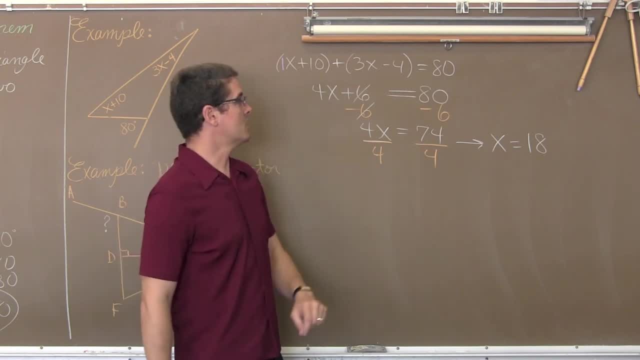 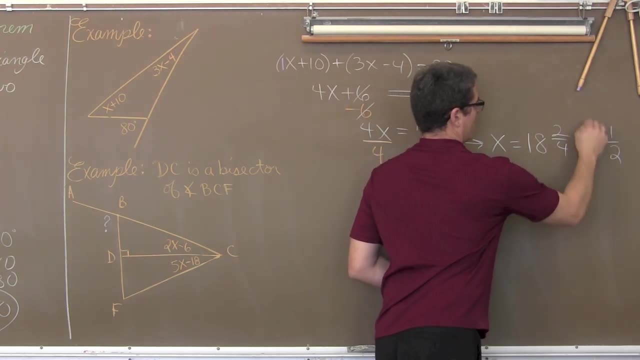 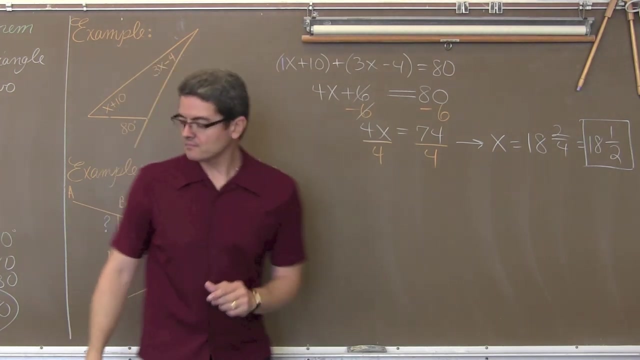 4 times 8 is 32.. So that leaves you with a remainder of 2.. So it is 18 and 2 fourths, or it is 18 and 1 half, and that is our value for x. Now over here, let me make sure that that is visible. 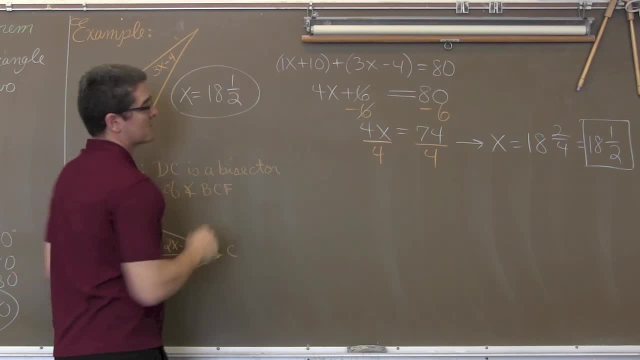 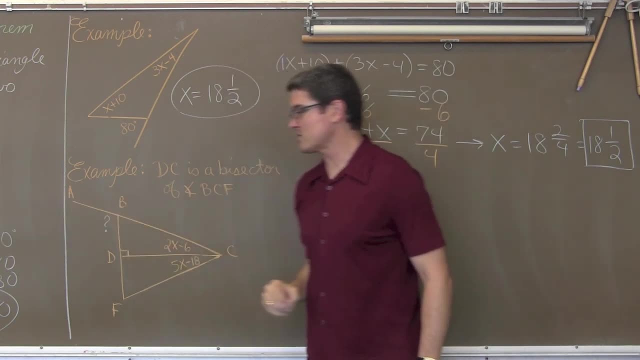 4 times 8 is equal to 18 and 1 half. That was our final solution. Over here we have a lot more going on. We have a couple of right triangles. We have an external angle extended on. We have dc is a bisector of angle bcf. 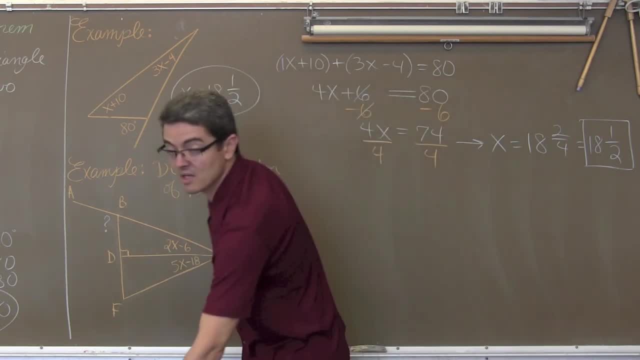 So dc is a bisector. I got some clouds coming in. it looks like I am a little dark. Let me pause this and brighten up the camera a bit, and that will give me a chance to make sure you can actually see all that work. 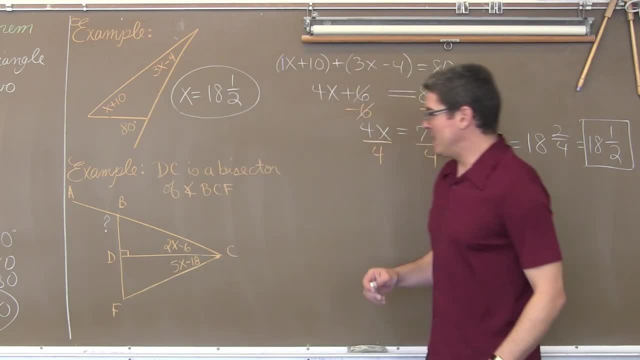 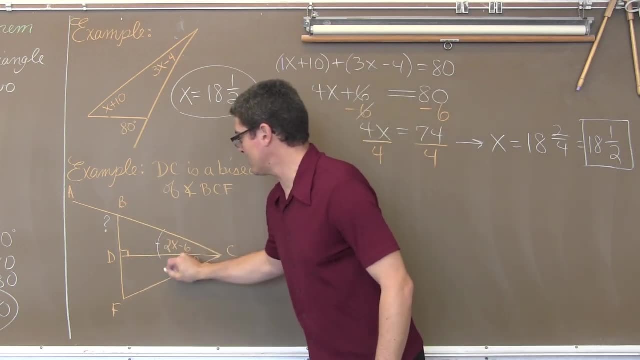 Alright, That looks a little better. Um, So if dc is bisecting angle bcf, then these angles are going to be equal And ultimately we are trying to find out the measure of this exterior angle. but I can't find the measure of this exterior angle until I know the measure of these two angles. 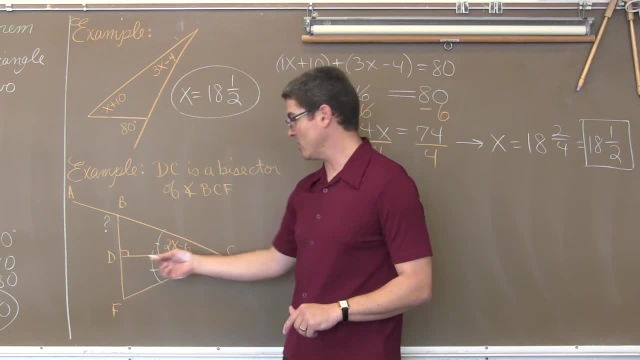 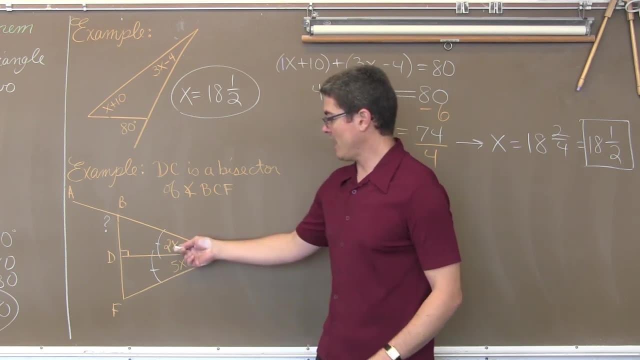 Now I know this is 90 because I had drawn a right angle notation in here, but I don't know what this angle is and I am not going to know the measure of this angle until we find out what x is equal to. Well, how am I supposed to solve for x so that I know how big this angle is? 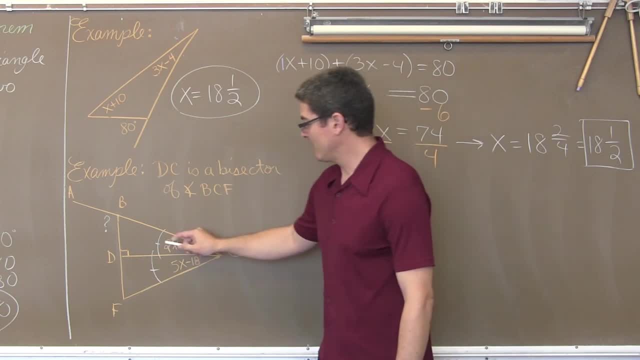 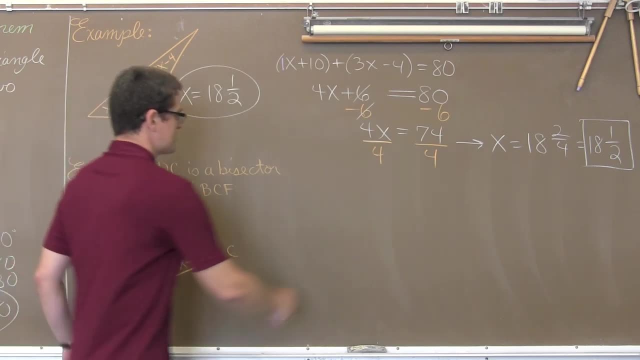 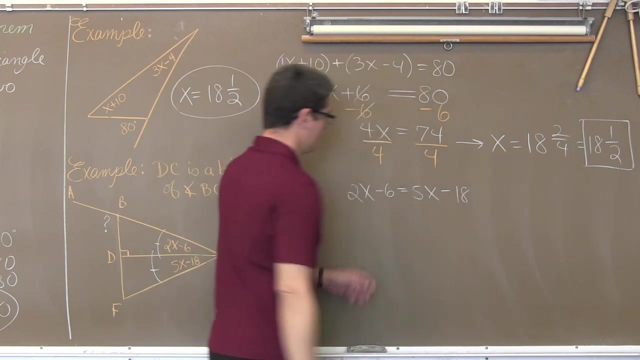 Well, I was told that dc was an angle bisector, so this means that these angles must be equal, and that is how I am going to solve for x. I am going to set these measurements equal to each other, So we have: 2x-6 is equal to 5x-18.. 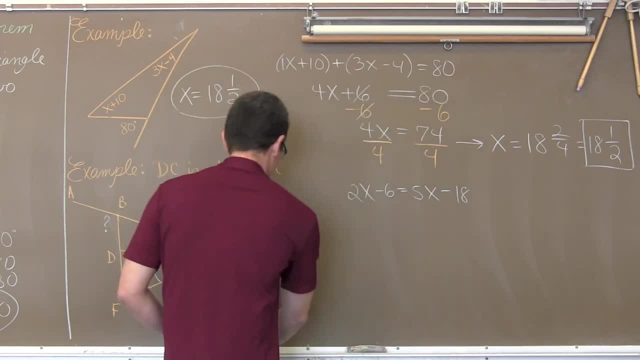 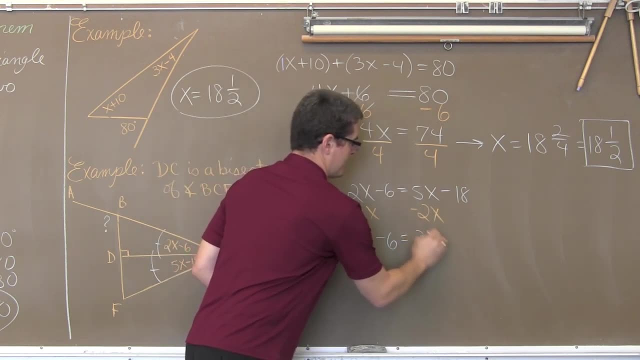 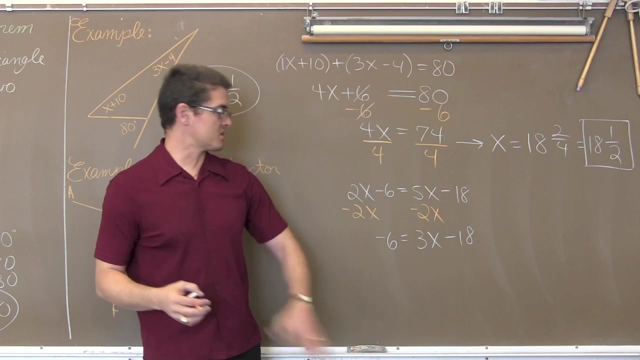 We are going to subtract both sides by 2x Sit well And um gives us negative. 6 is equal to 3x minus 18.. Now I put my variable on the right hand side. Some students unfortunately make more mistakes when they move their variables to the right. 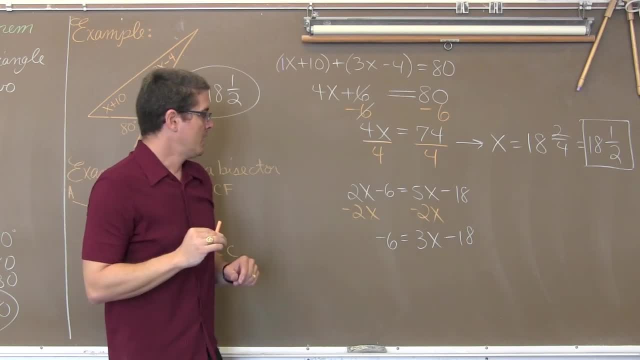 because they are so used to the variable being on the left and all the numbers going to the right. But if I subtracted both sides by 5x I would have created a negative answer in front of my x, and that should not be a problem either. But you know I see mistakes happen. 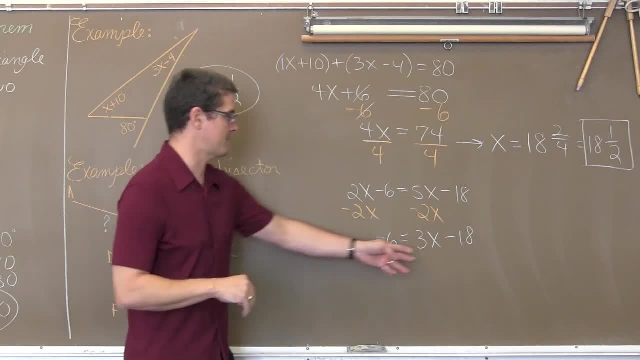 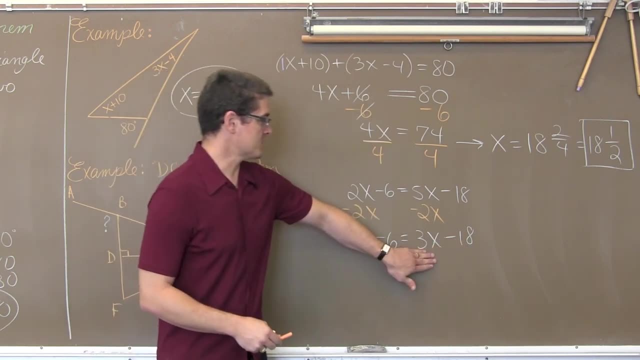 when you create more negative numbers as well, So do whatever works best for you. It doesn't matter what side of the equation you put your x on. Well, now my x is on the right, so I am going to start moving everything to the left Over on the right hand side of the equal sign. 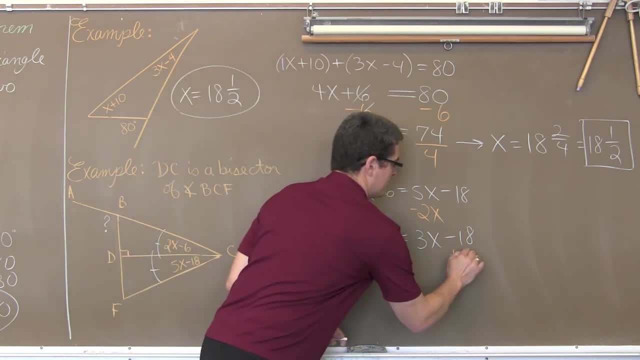 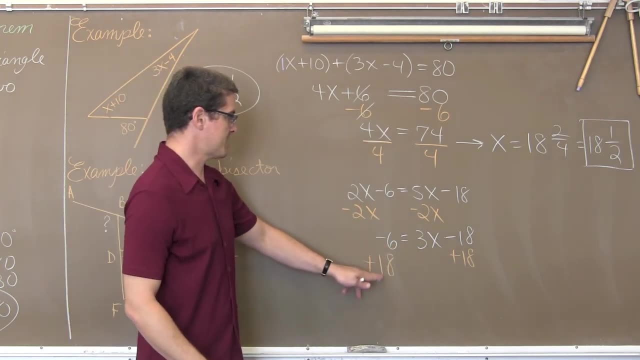 I have a negative 18.. I am going to get rid of that. I am moving it from the right side to the left, which means I need to do the opposite math operation. So negative 6 plus 18.. That is 18 minus 6 basically, which is going to be 12.. 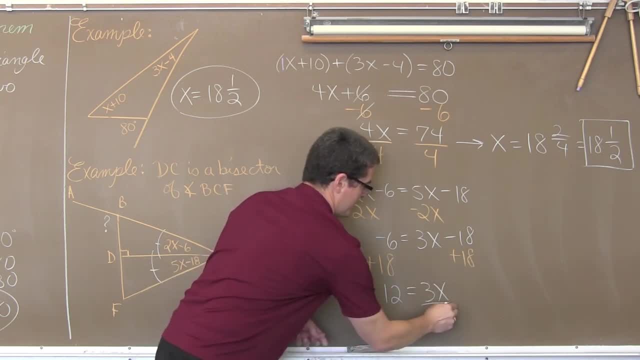 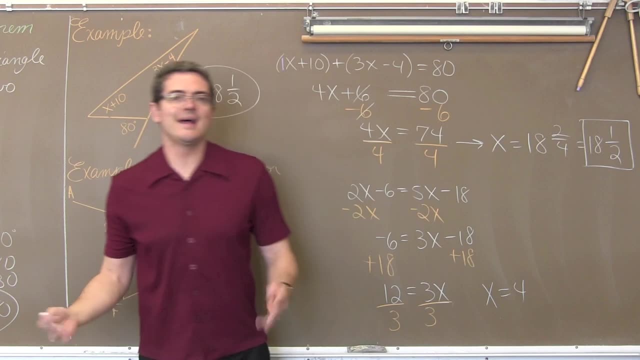 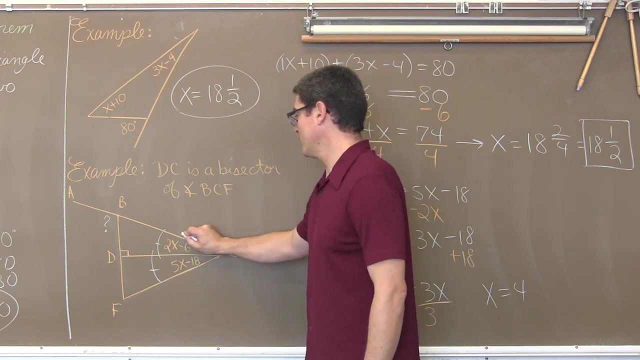 Subtitles by the Amaraorg community equals 3x. Divide both sides by 3 and we get that x is equal to 4.. Well, x is not an angle measure. x is part of this expression. So if I come back up here, I have looking at. 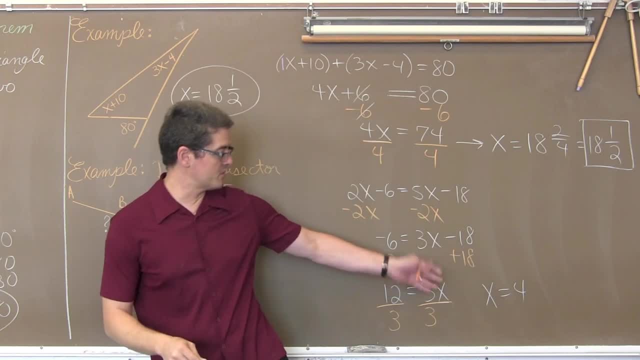 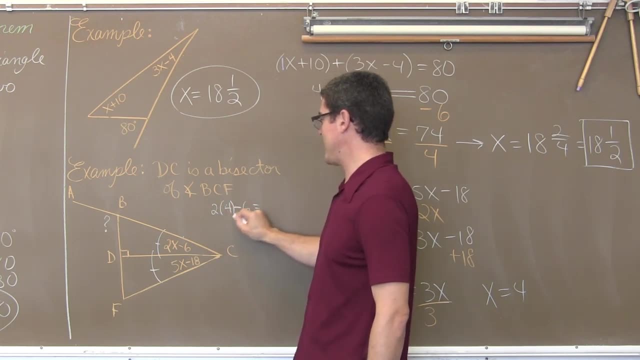 this expression: I have 2 times x, which we just found was 4 minus 6.. So 2 times 4 is 8 minus 6.. So 8 minus 6 is equal to 2.. So actually this angle measure is very, very small. 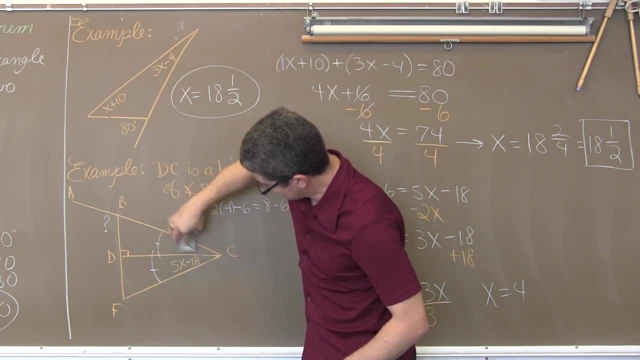 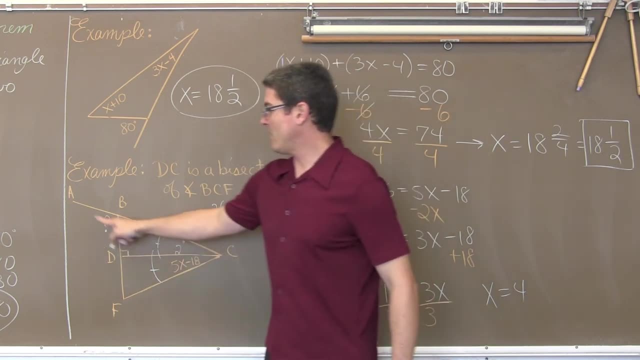 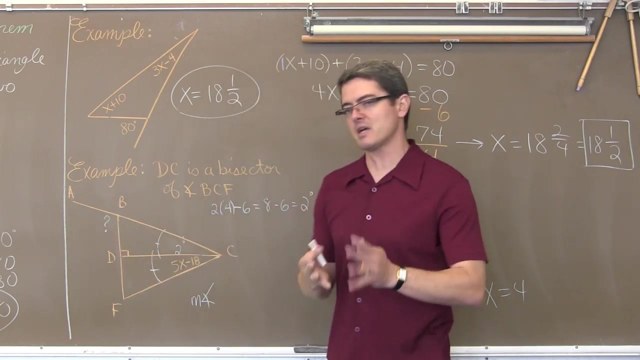 It is actually only equal to 2 degrees. So let me take this expression out and put the actual measurement that it is equal to, which is 2 degrees. Now, how much is, or what is, the measure of angle? either dva or abd. Just make sure you put the vertex in the middle. So, 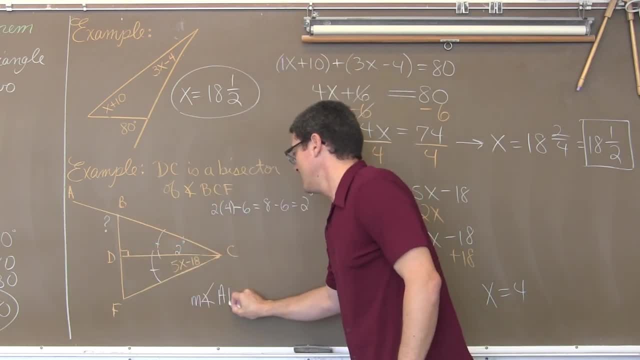 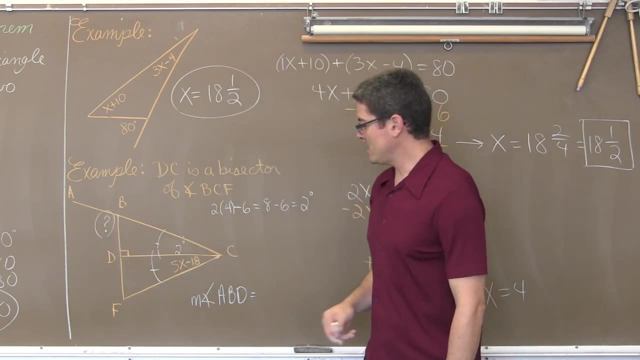 I am going to call it abd, The measure of angle, abd. Let's write that down. So this is the question mark. I hope I made it clear enough. that is what we were looking for. It is equal to the sum of. let's see, this is the external angle I am dealing with. This is the adjacent. 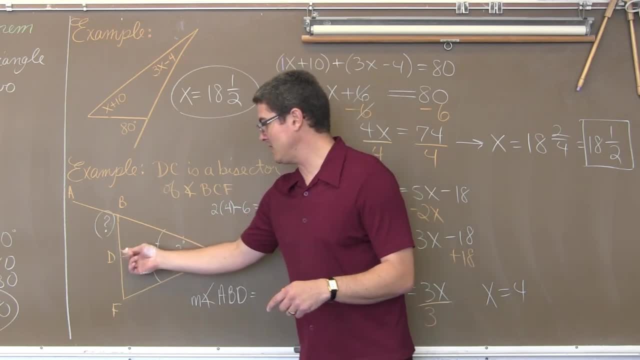 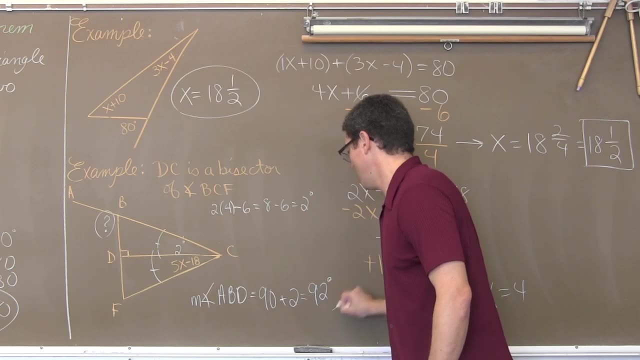 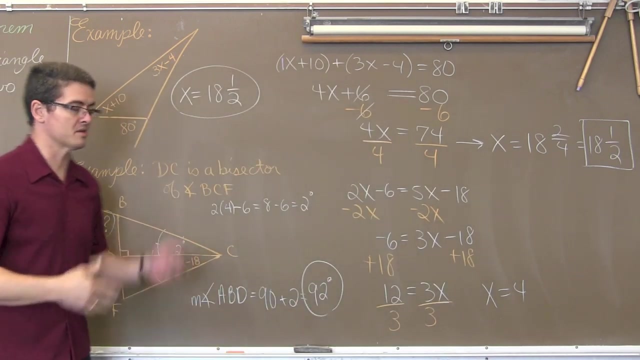 interior angle, That is not the remote interior angle. It is 90 plus 2.. So it is 90 plus 2.. So my external angle is equal to 92 degrees. This, hopefully, with your geometry book, would be maybe sort of towards well, one like this. of course, This is what was in my book, But